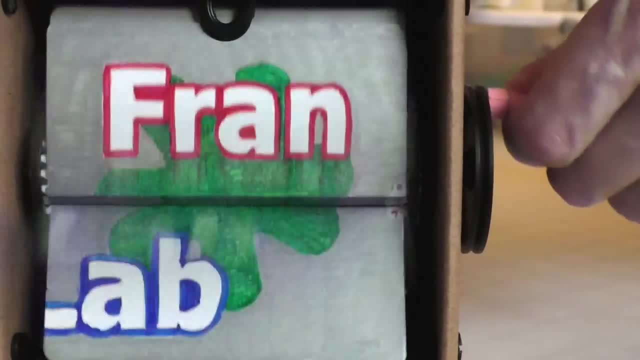 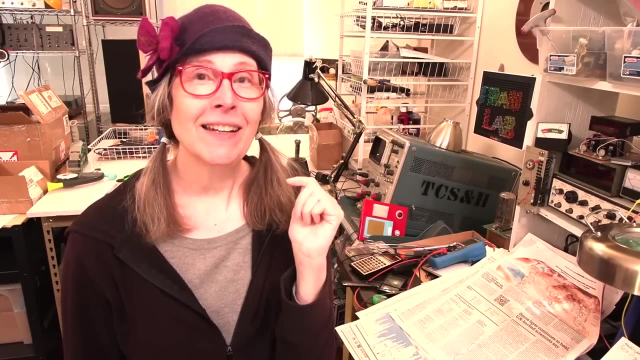 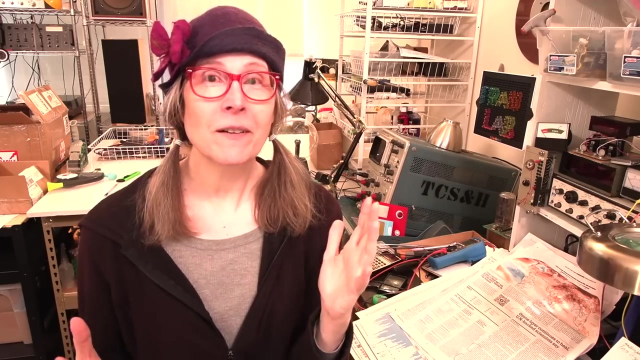 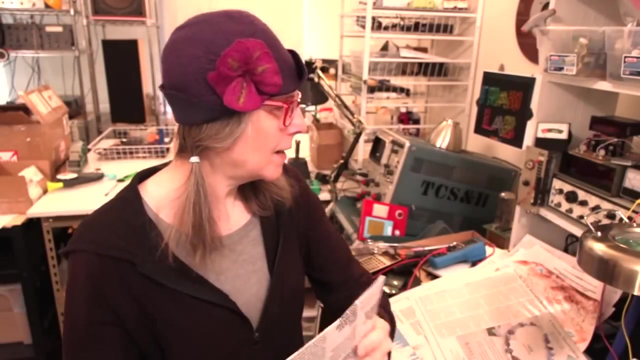 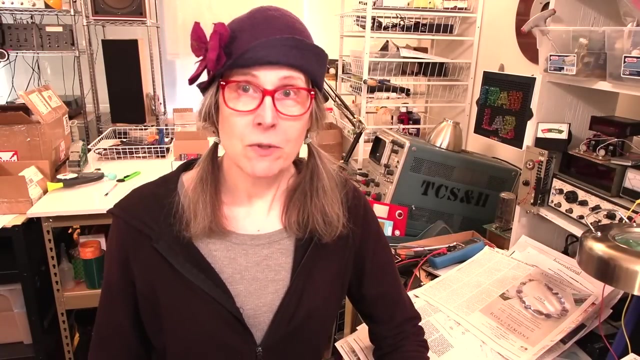 Okay. Hey, it's Fran in the lab again with some good news for once about the atmosphere. Yeah, it was in the paper. Ozone layer continues to heal, UN-backed scientists say. And another one: ozone may be fully restored in decades. You probably didn't hear about this, but it. was big news to me. A study just published by the World Meteorological Organization says that at the current rate, the ozone layer could recover to 1980s levels across most of the globe by the 2040s and by 2066. in Antarctica, which is where the big hole is, It fluctuates. with the seasons, but the hole in the ozone layer is still there. The ozone layer is most prominent over Antarctica. Scientists said that the latest ozone data and projections are nonetheless further proof of the success of the Montreal Protocol, the global 1987 agreement to phase out production and use of ozone-depleting substances mostly. 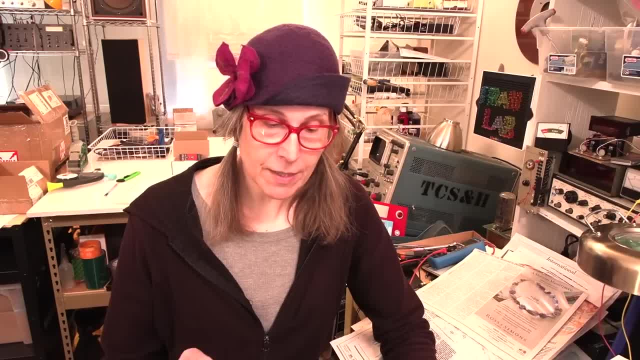 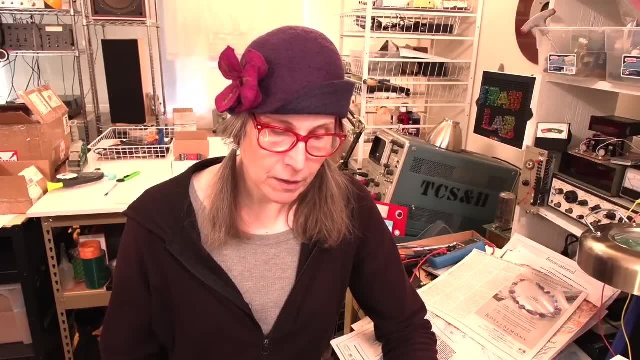 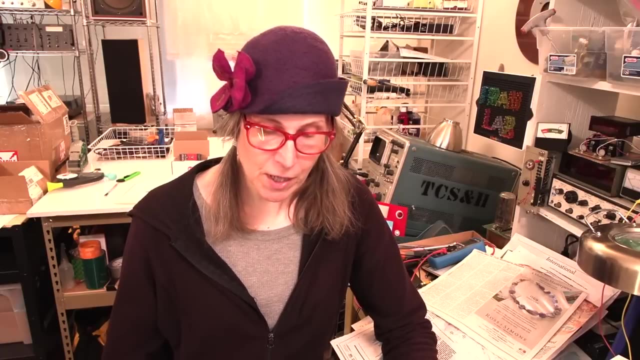 chlorofluorocarbons, CFCs, And it goes on to say that a recent decline in observed levels of the chemical known as CFC-11, in particular, which as recently as 2018 had been observed in higher than expected levels and traced to manufacturing in China. but it goes on. 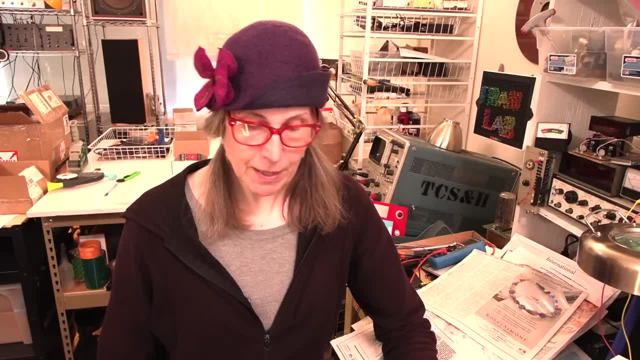 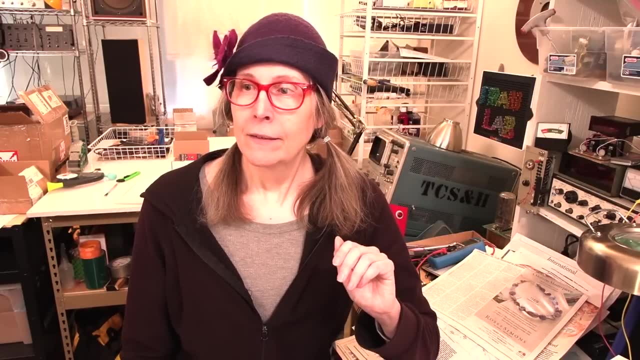 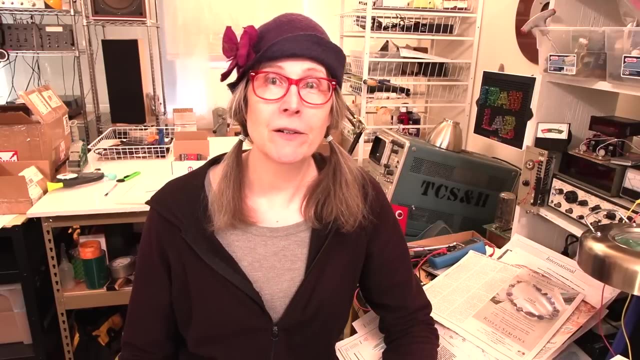 to talk about the ozone, how ozone is created and everything. I'm going to get into that. But yeah, this is good news, And this is case and point, that we can make decisions that can change our situation for the better as far as the atmosphere goes, The ozone layer. 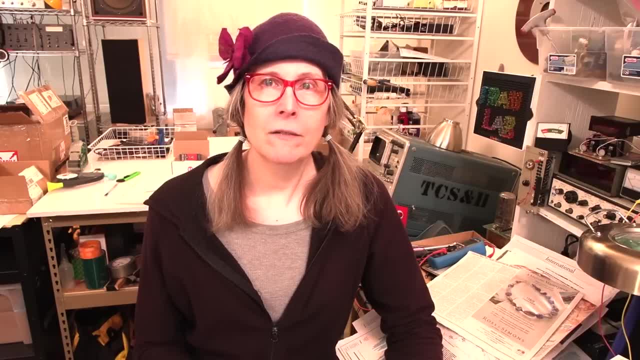 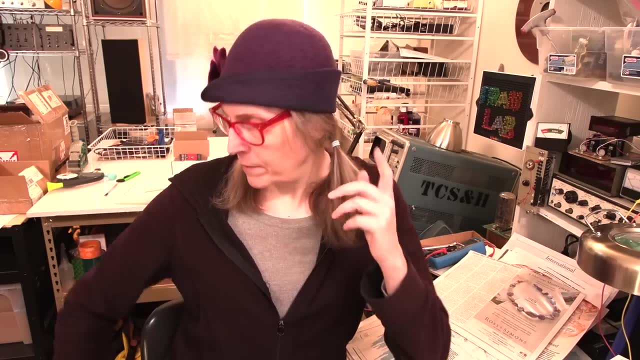 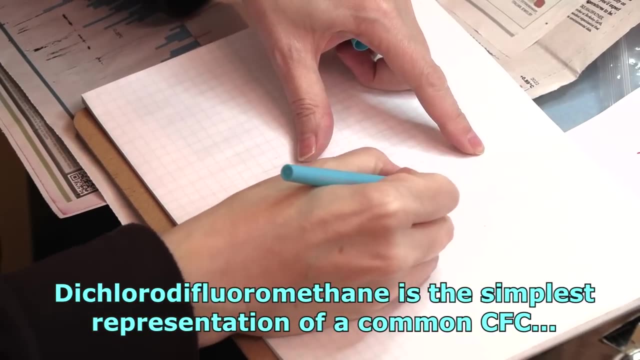 depletion. it resulted from the production of chlorofluorocarbons on an industrial scale for many decades, The reason being that? chlorofluorocarbons- I'll show you, Let's go to the bench. So yeah, chlorofluorocarbons, it's a very stable molecule made up with a single carbon. 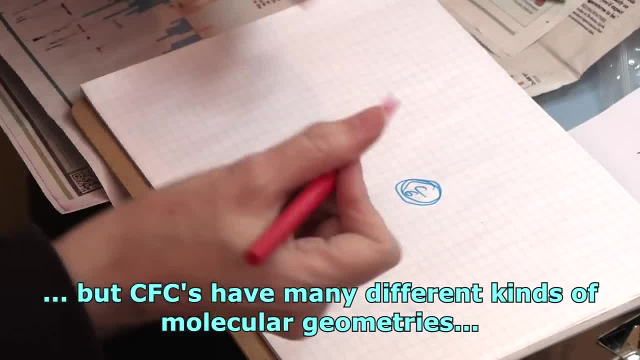 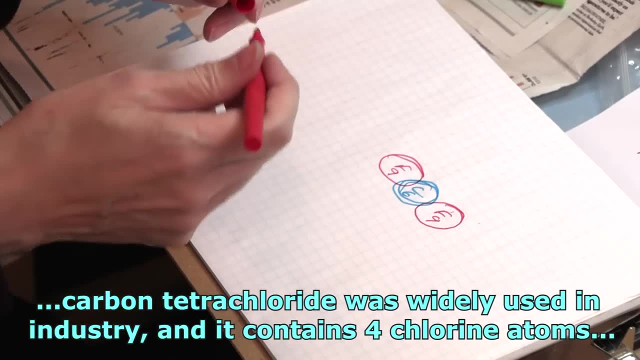 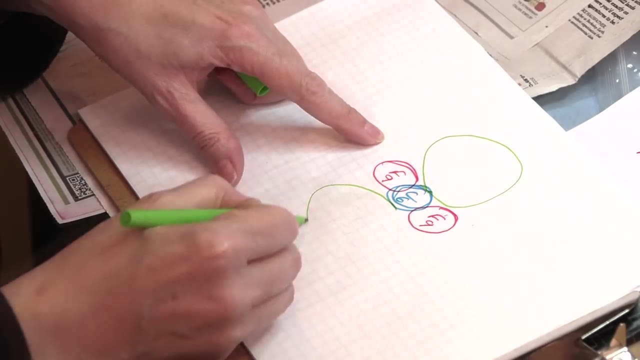 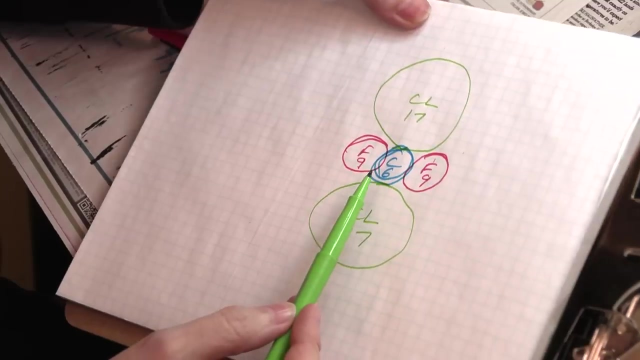 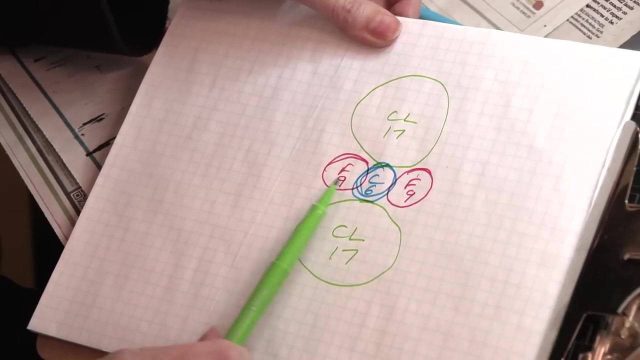 atom atomic number of six. it's got two fluorine atoms right. atomic number of nine and two, two chlorine atoms like a molecule. that's kind of like this: So the carbon and the fluorine atoms, they're just about the same size because they occupy the same outer level of valence. 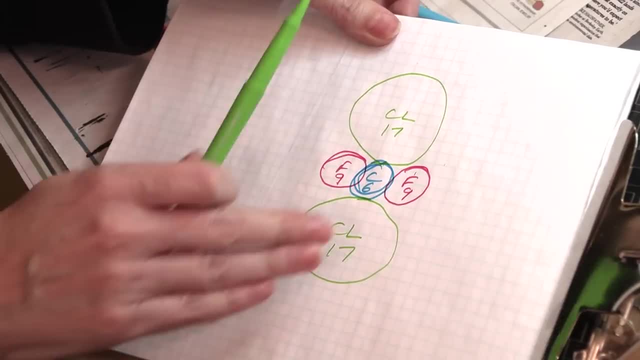 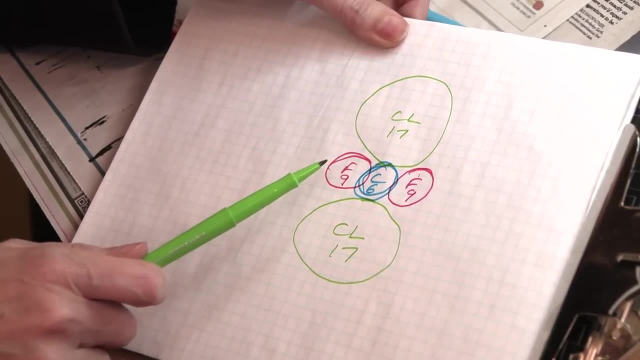 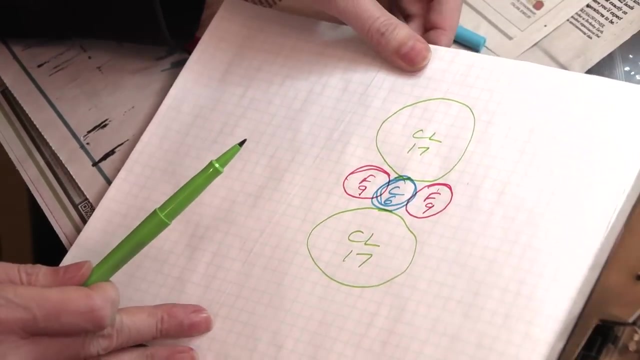 electron, you know the same level, shell, The chlorine atom, much larger, much heavier and in regular conditions this is an extremely stable molecule And, because of the molecular geometry of the chlorofluorocarbons, made them ideal pressurants and refrigerants. So these 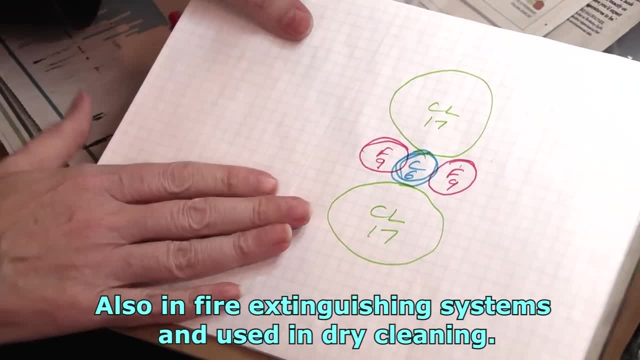 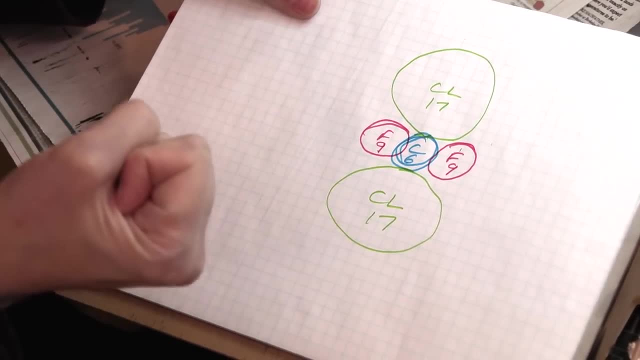 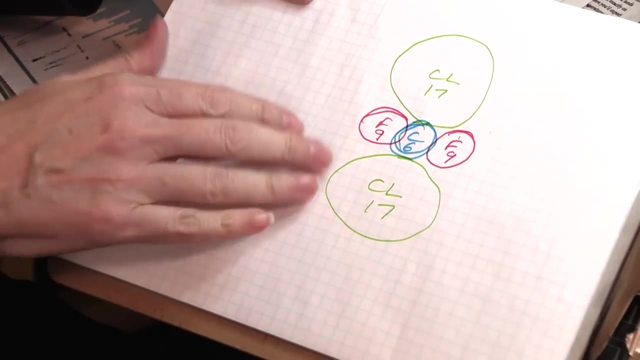 were used in refrigerators, air conditioners, because this kind of molecule, the geometry of it, it could be compressed to a very high degree and then it could release all that energy. It was a perfect refrigerant, And what made it an? 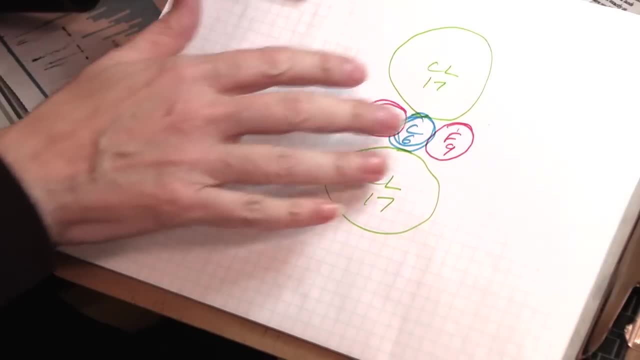 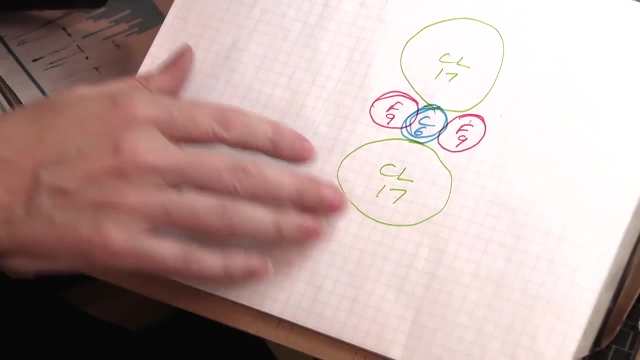 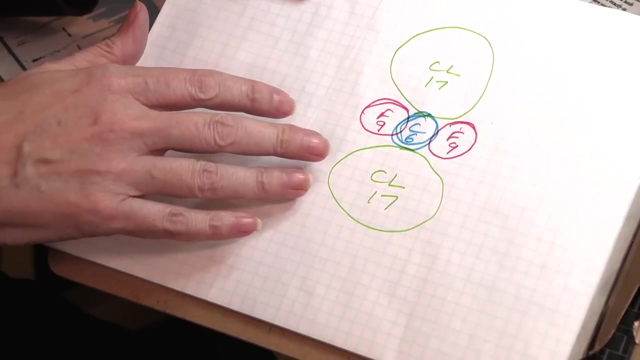 ideal pressurant for aerosols is the fact that it is so stable. It is non-reactive, So you could put a molecule like this in abundance in a container as a pressurant, along with just about any other kind of solution or compound, and it wouldn't react. So chlorofluorocarbons: they were one of. 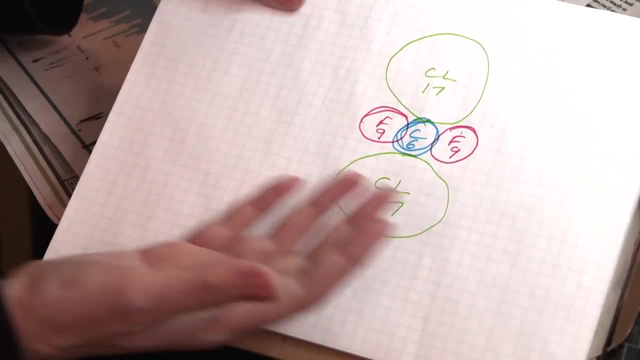 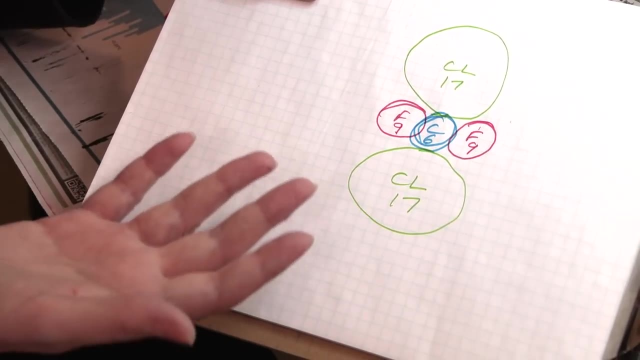 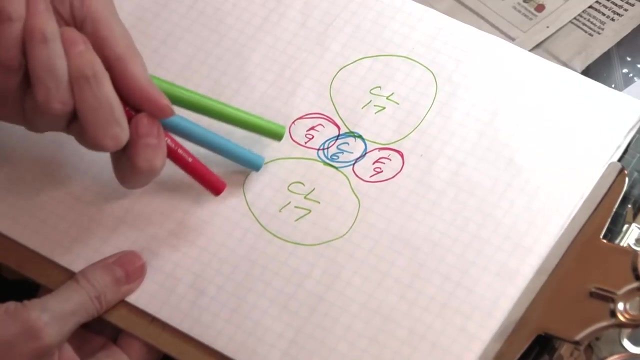 the miracle chemicals And as far as like human interaction, it's pretty much like a benign chemical. It doesn't have any chemical reactivity. It's odorless, tasteless, colorless, So it really didn't raise any flags at all, The CFC molecule. it was behaving very differently in the stratosphere. 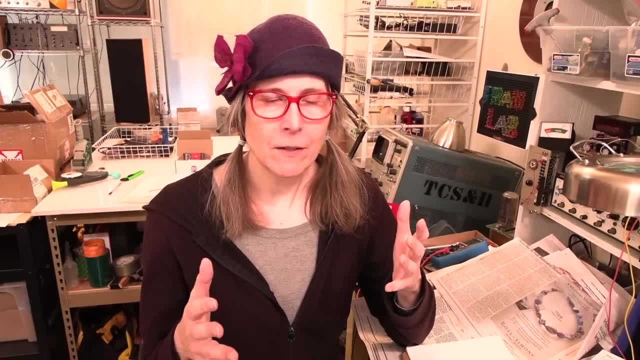 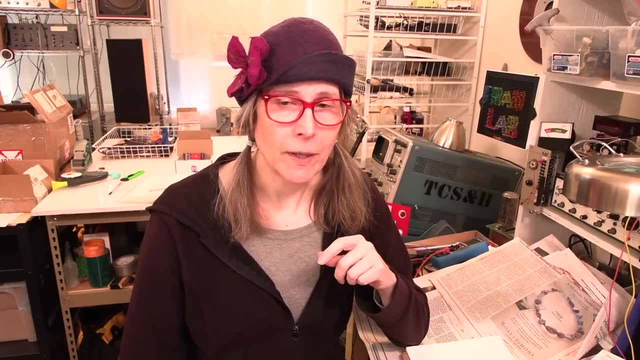 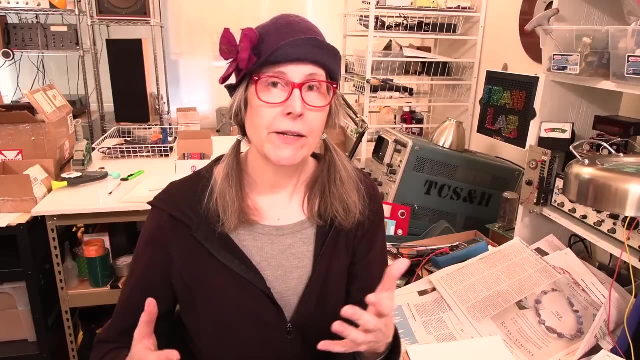 So this is where it gets into the interaction of ozone and really what ozone is and how it protects us And why do we even need an ozone layer anyway. Well, ozone is created from the interaction of ultraviolet radiation and the atmosphere. It happens in the stratosphere, which is the layer of the atmosphere where molecules get close enough together that the atmosphere becomes sensible. Above that, it's so rarefied that it's really just where meteors burn up and where you get drag in the very high atmosphere when objects are starting to reenter. 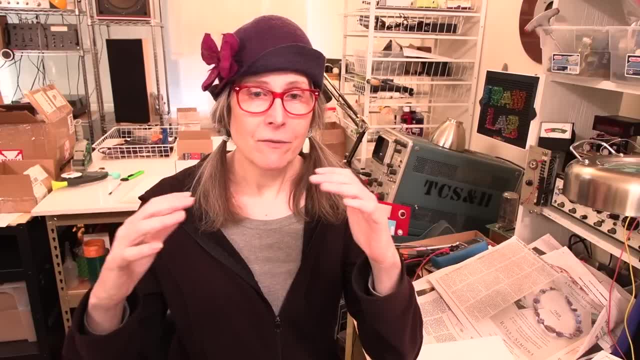 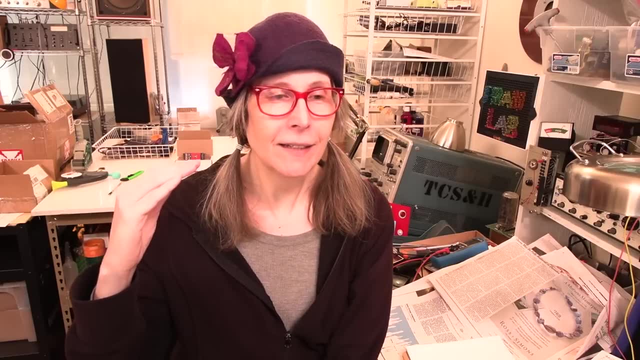 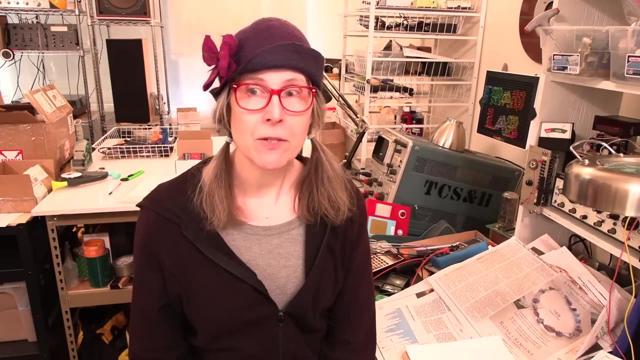 the atmosphere. But you know, the stratosphere is the beginning of the really sensible atmosphere And so it is where ultraviolet and oxygen interact Really for the first time. There's lots of fine print to this and I'm not going to get into the deep chemistry and interaction of things You can certainly. 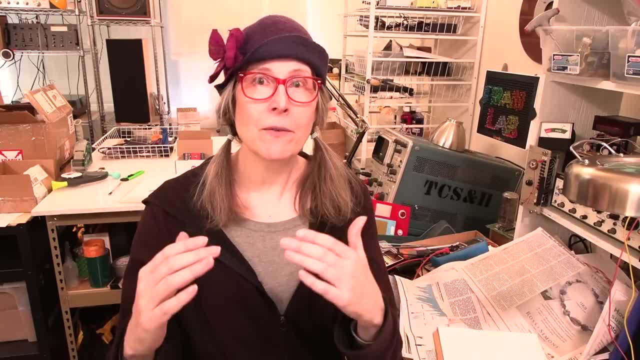 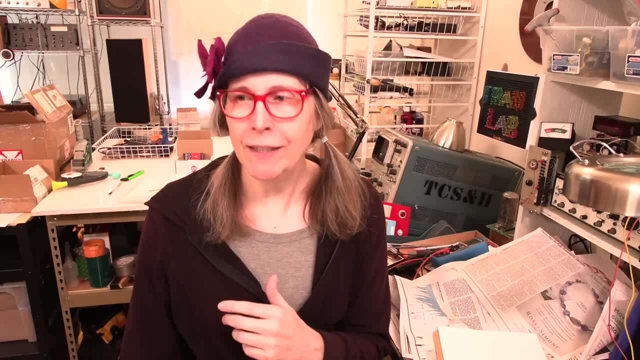 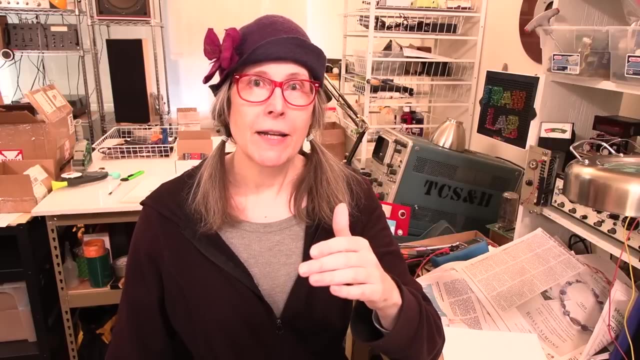 You can certainly read about it at your leisure. But you know, in the upper atmosphere, in the mesosphere, the thermosphere, Ultraviolet radiation creates something that's called hot oxygen, oxygen, which is that's a different topic. But in the stratosphere, where ultraviolet radiation UVB, UVC and the vacuum. UV begins to run into oxygen. to really understand why we have an ozone layer, we have to realize that the atmosphere did not always contain oxygen. The early Earth for well. for billions of years it was mostly methane and ammonia, with some other trace gases. And photosynthesis is responsible for putting the oxygen into the atmosphere that we as mammals can breathe. It's only been since we've had molecular oxygen in the atmosphere in abundance that we've had ozone. So in the highest levels of the stratosphere, where oxygen molecules, O2,. are bombarded by ultraviolet radiation, they begin to transform, because oxygen is easily ionized by UV And the specific frequency of the ultraviolet radiation is going to determine exactly what happens to that oxygen molecule. So there's two gases in the stratosphere. primarily it's N2. 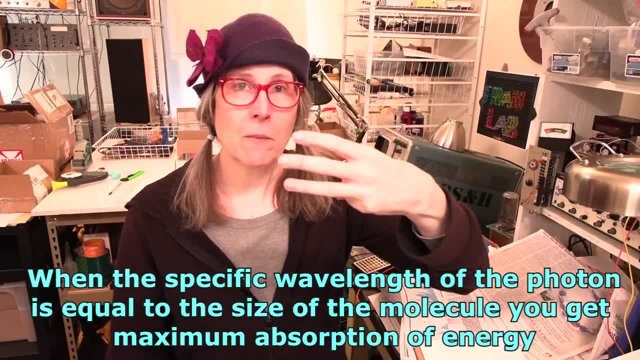 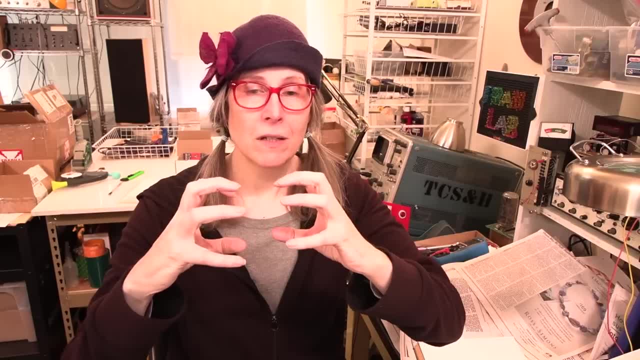 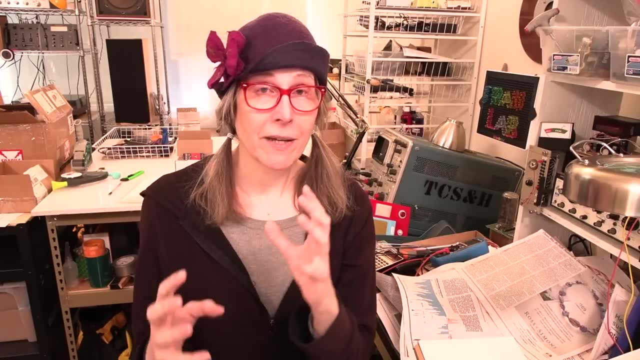 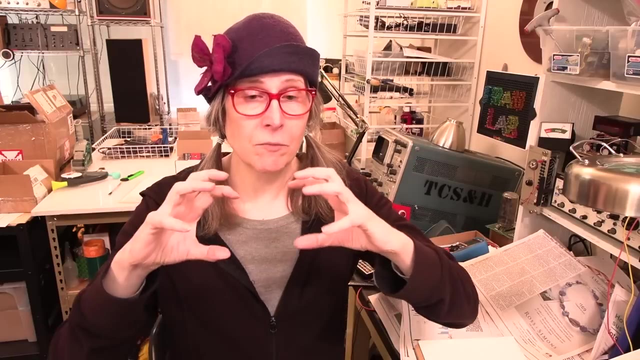 and O2.. N2,: it's a triple atomic bond, three electrons shared by two nitrogen atoms. It is one of the most most unbreakable bonds on the planet. Ultraviolet radiation will not break up nitrogen molecules but oxygen. O2, shows a duplex bond- two electrons, and it is easily ionized to the point of. 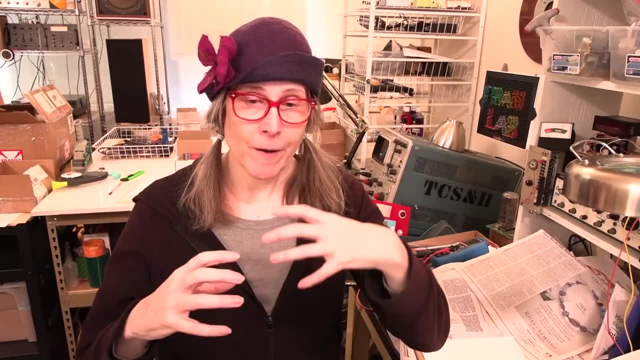 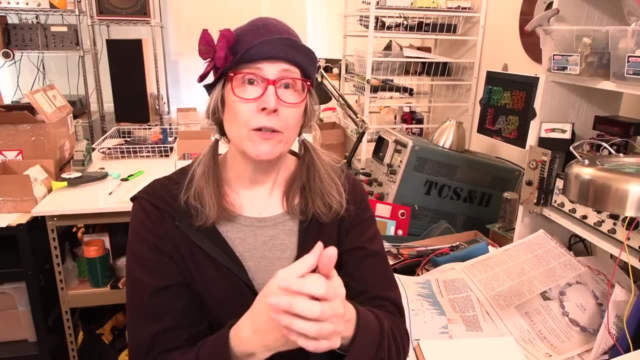 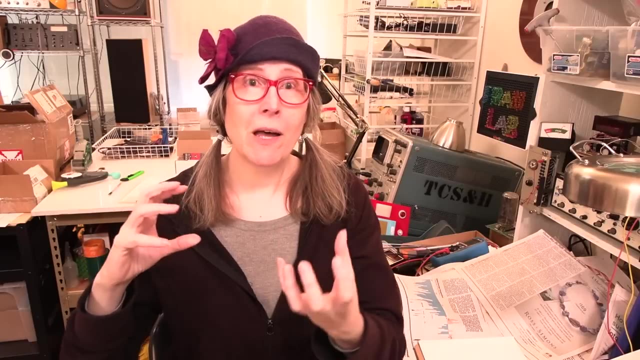 breaking apart in the upper atmosphere, And so there's a complex process that goes about where far UV, like the vacuum UV, UVC will obliterate oxygen molecules into free oxygen molecules, And so the hydrogen ions, which will then readily bond with other oxygen molecules and create O3, sharing two. 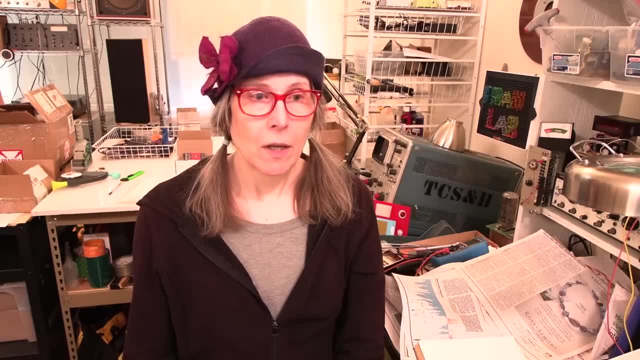 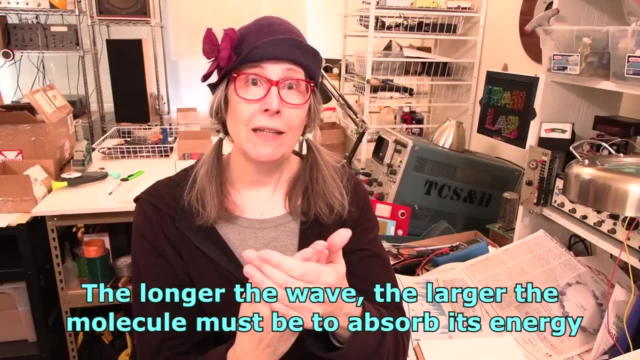 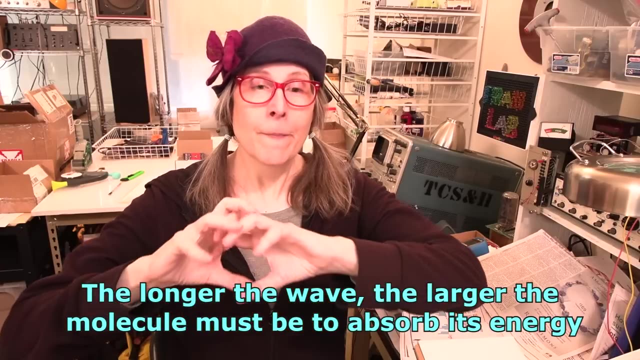 electrons with three oxygen atoms, And that configuration then is easily absorbed by UVB, which when UVB hits an ozone molecule, it easily breaks that bond and transforms its energy into breaking that extra oxygen atom off the ozone and making it free of the oxygen molecules. And so that's one of the things that we're. 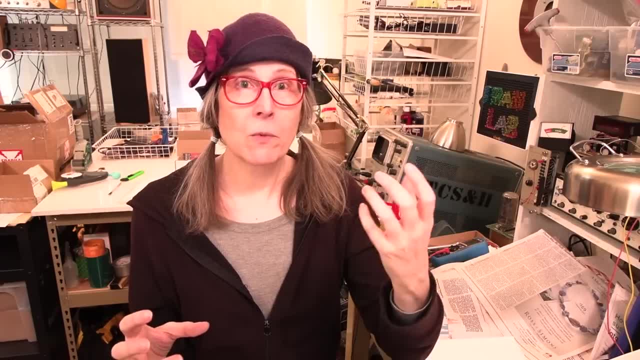 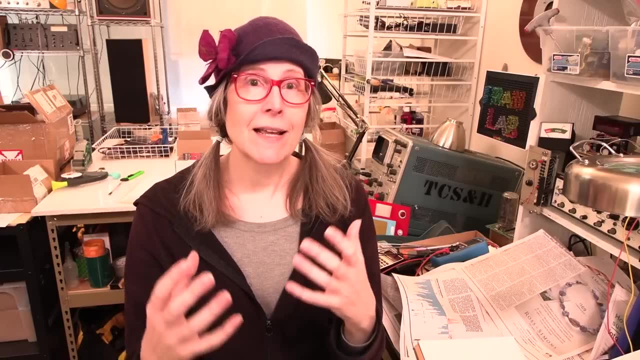 going to talk about in the next lecture. Now we're going to look at the difference between UVB and O3 to combine with another O2 molecule somewhere else and in the process it loses energy and gets absorbed completely, And it is through this process that the really dangerous UV. the ionizing radiation, gets absorbed by this layer of the atmosphere. The far UV gets absorbed by breaking up O2 molecules and O3. And then the UVB gets broken up by being absorbed by O3. So the real problem with not having the ozone there is that the UVB gets through. It doesn't get absorbed by O2.. It just gets refracted And we end up getting a lot more UVB on the surface where it can break our molecular bonds in our biology. So the thing about it is organic. chemistry is based on carbon and organic molecules. 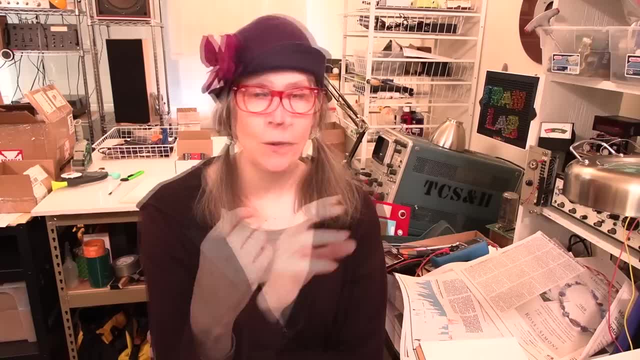 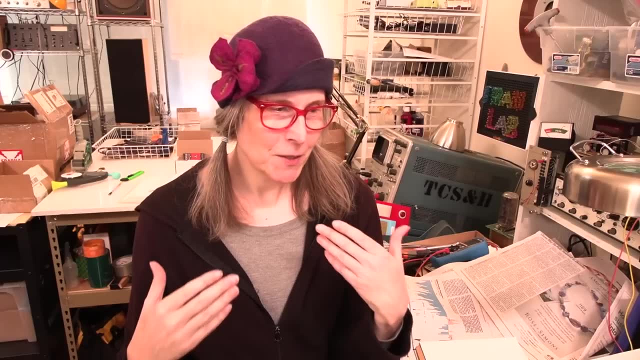 And the reason that organic chemistry works is that the bonds are so easy to break, which makes it so dangerous for us as a species, in the long term, to be exposed to UVB, And so it was in our best interest to restore the ozone layer. 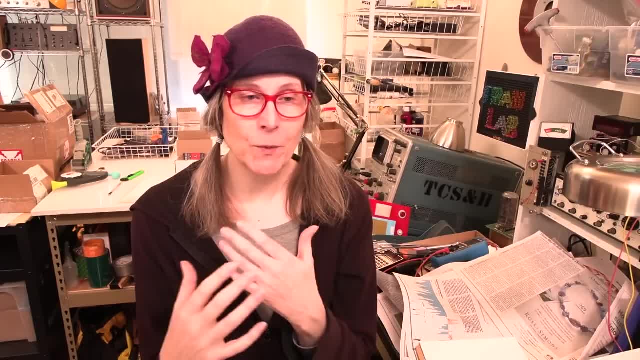 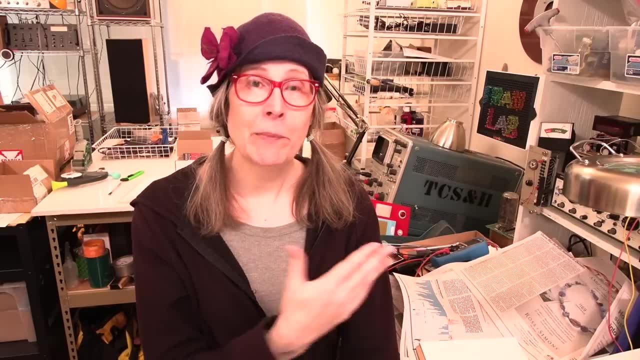 to get ozone levels back up to pre-industrial levels so that we could reduce our level of skin cancer and other things. So what is it about chlorofluorocarbons, this very stable, miracle chemical that created a problem with the ozone layer? 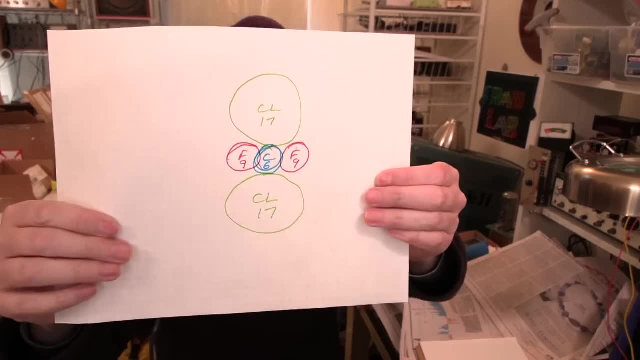 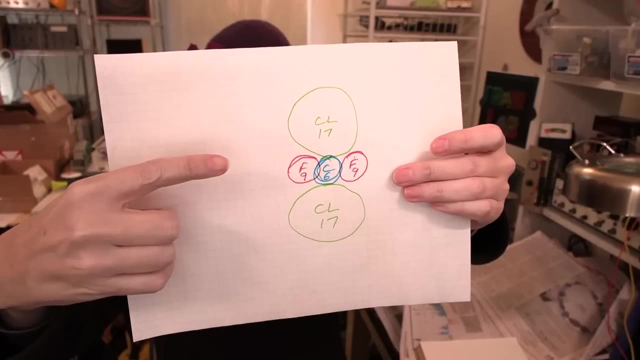 Well, the issue really comes down to the chlorine atoms, Because in the CFPB I see, the chlorine atoms are much, much larger and much, much heavier than the carbon and fluorine atoms. And in chemistry, when molecules break down, the largest atoms with the weakest bonds are going to be the ones that are going to be broken first, And the chlorine atoms. they're very easily broken off of the chlorofluorocarbon, with a minimum amount of energy, And UVB, which is typically absorbed by the ozone layer. 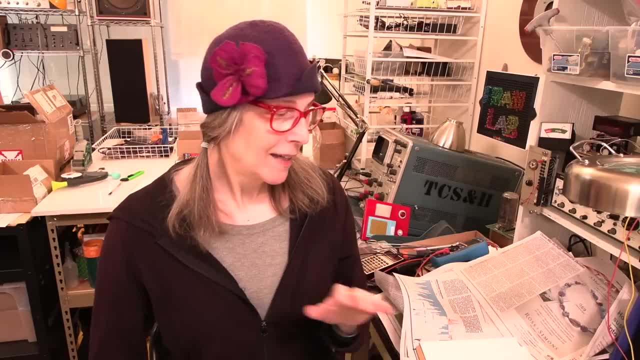 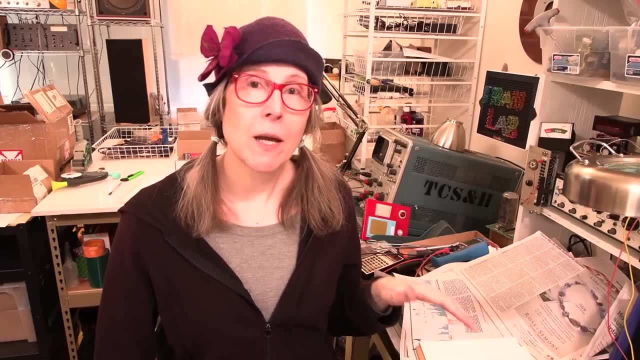 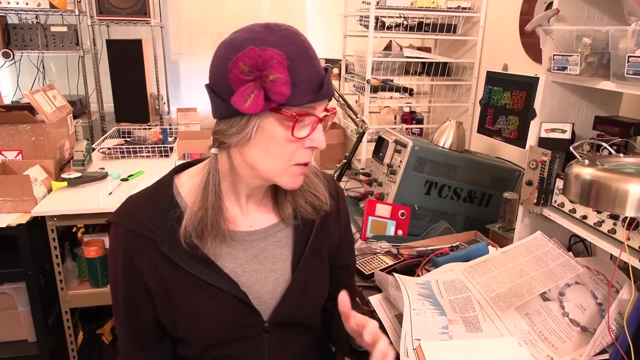 by breaking up ozone molecules, it very easily breaks the chlorine atoms right off the chlorofluorocarbons, And so when these chemicals got into the upper atmosphere, raising to the top of the stratosphere in any kind of concentration, it created this chain reaction process where the chlorine atoms were being 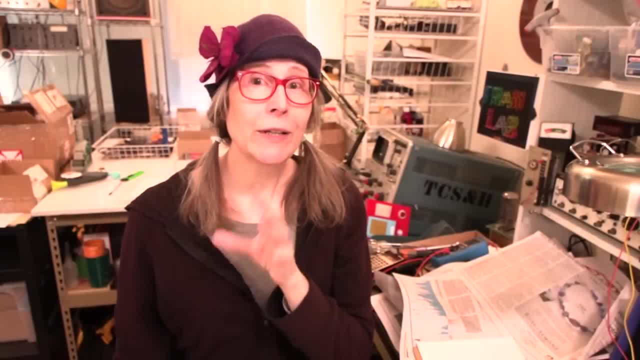 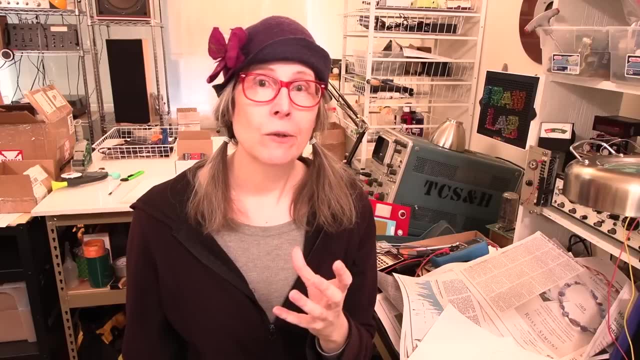 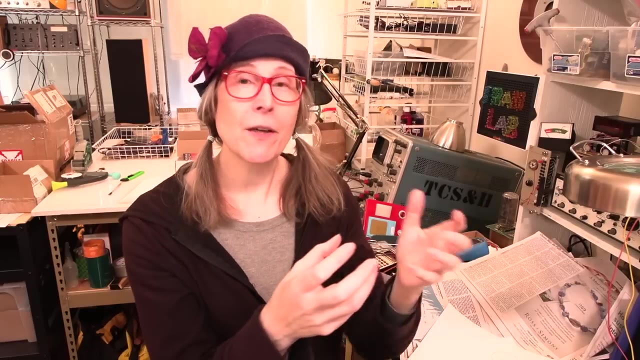 knocked off of the chlorofluorocarbons, creating free chlorine gas And, once in the atmosphere, the free chlorine it was. it was destroying the ozone by pulling those extra oxygen atoms off the O3 and recombining them with other oxygen atoms that have been pulled off of other ozone. molecules and recombobulating them into O2 and then just breaking free and being free chlorine atoms again creating this catalytic process of converting the ozone to O2, like on an ever-increasing scale, So that the natural process of ozone production by the far ultraviolet was being countered by the chlorine gas. 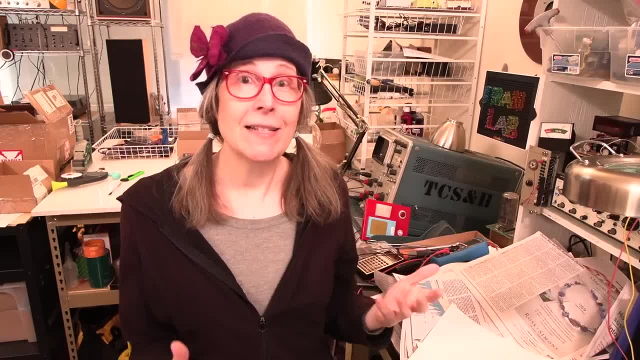 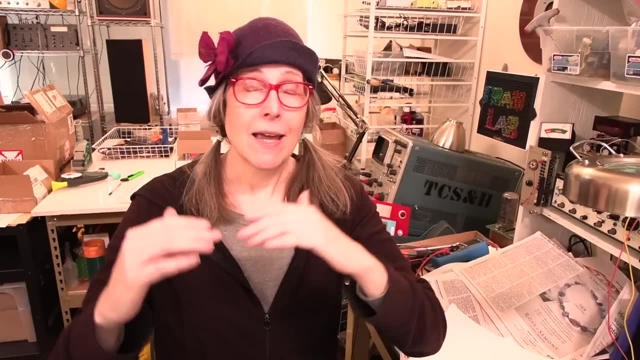 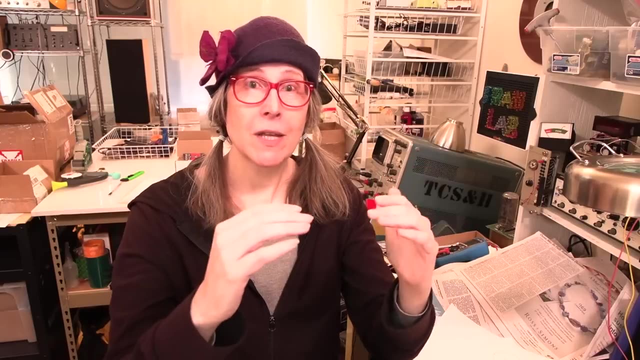 which is accumulating in the stratosphere from the ionization of chlorofluorocarbons, And it was creating this very slow, steady tipping of a balance that had existed for billions of years in the atmosphere, to cause the levels of ozone to reduce. 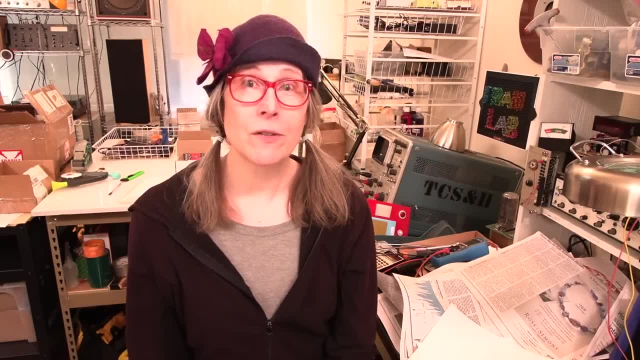 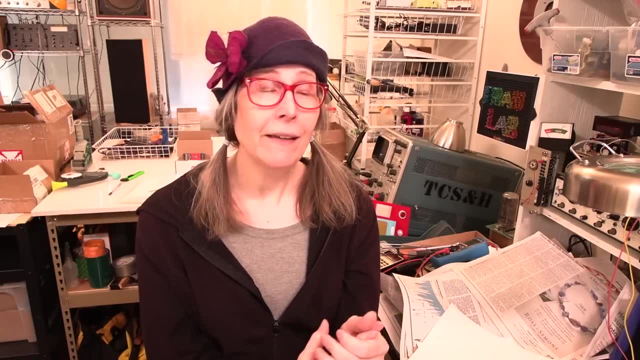 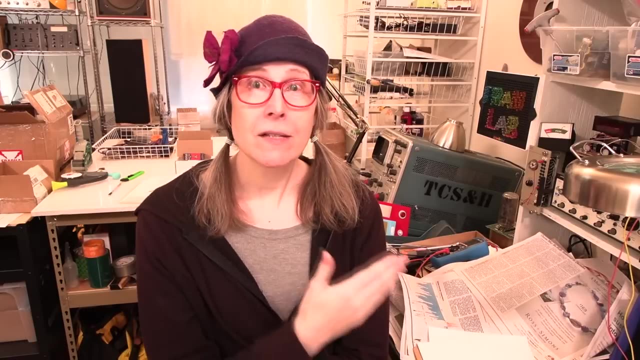 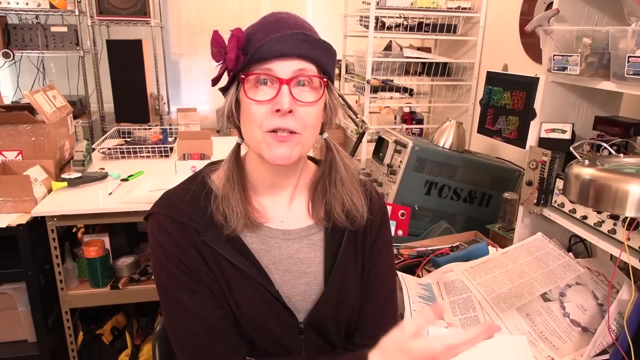 And those increasingly reduced levels of ozone were were creating pockets and holes in the ozone layer, which was allowing larger and larger amounts of UVB to come through, And this was the concern and the reason for the Montreal Accords. So this is a case and a point of a situation where we made a mistake by creating a situation which we did not foresee. 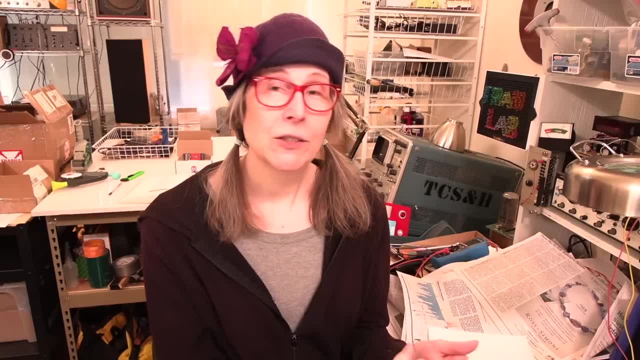 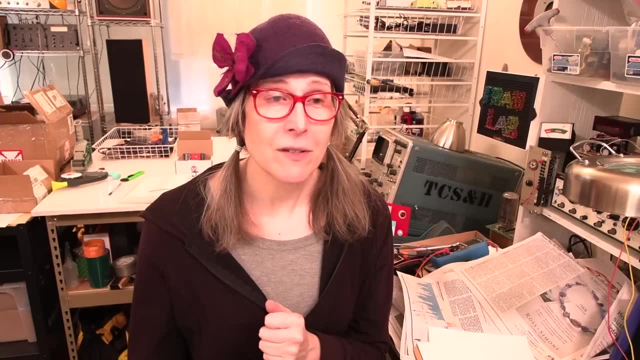 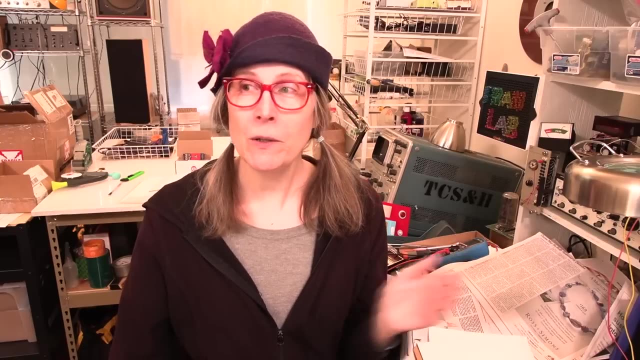 We looked at the data, projected a future that we didn't want to have as a species. made hard decisions worldwide to get rid of a chemical which made our lives so much easier and was really a miracle in so many ways. found ways to replace that chemical. 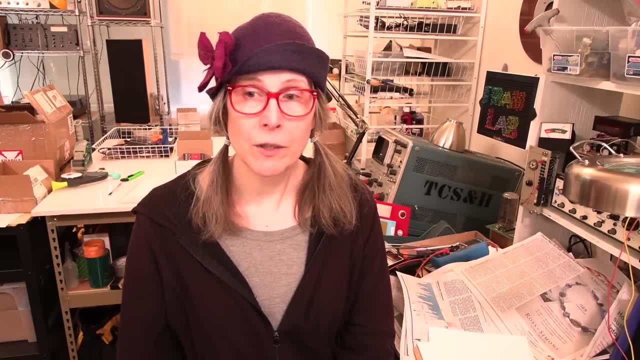 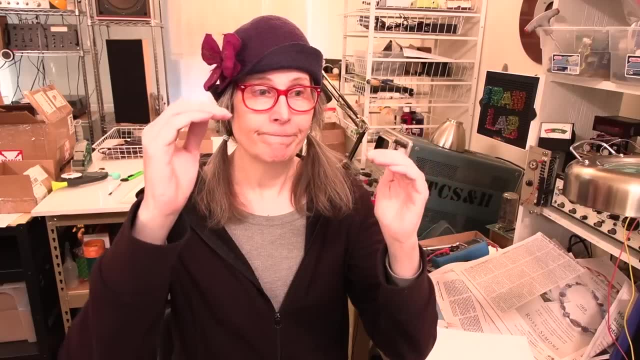 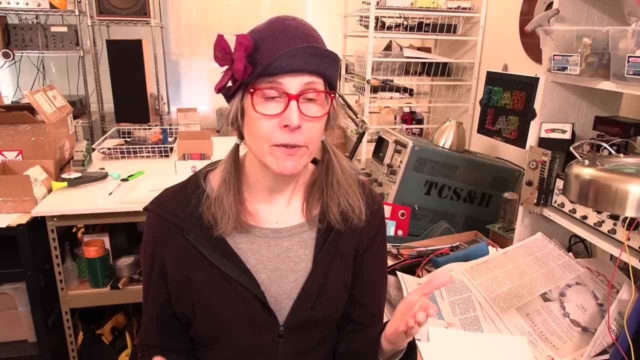 reduce and eventually pretty much eliminate its industrial use. and here we are, not even 40 years later, and we're seeing that seesaw begin to move in the direction we want. And once we stopped putting chlorofluorocarbons into the atmosphere on a massive scale. 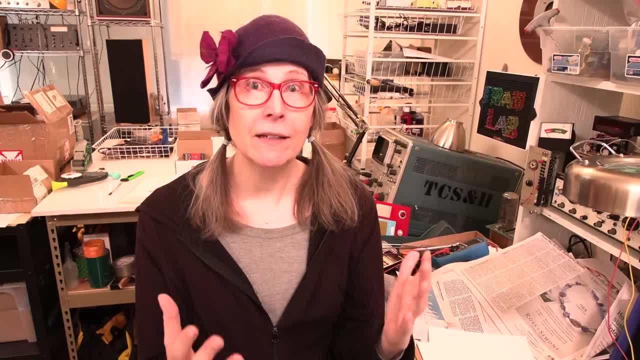 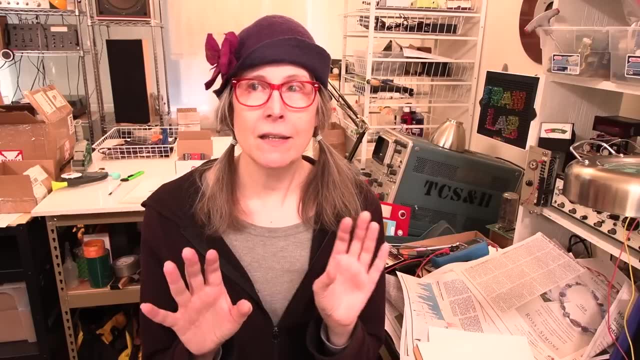 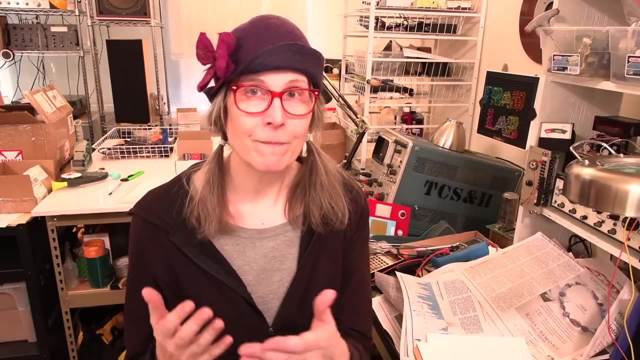 natural processes were just going to eliminate it gradually from the atmosphere, And we're beginning to see this. So this is the light at the end of the tunnel as far as climate change, And so we have to go from this to talking about the other elephant in the room, which is CO2.. 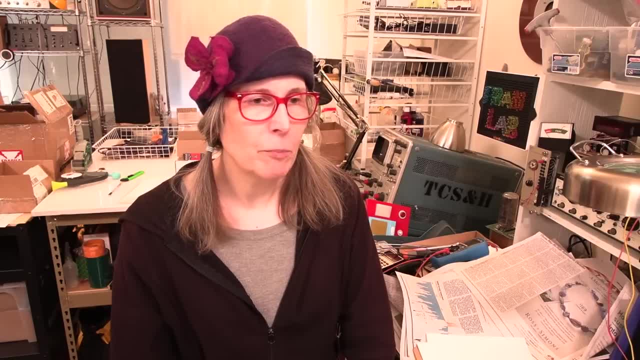 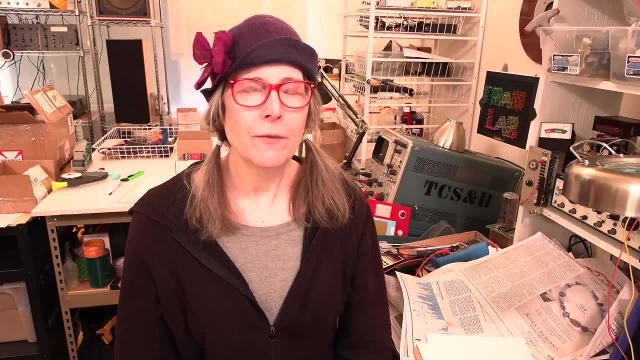 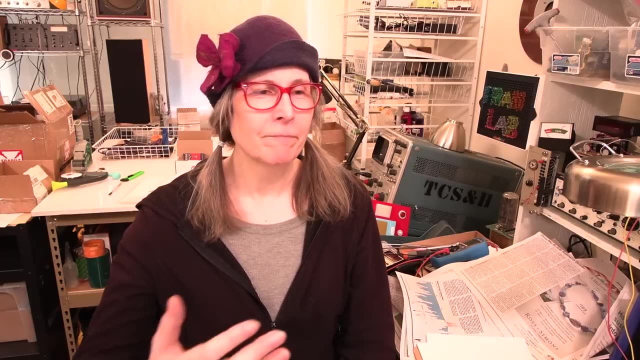 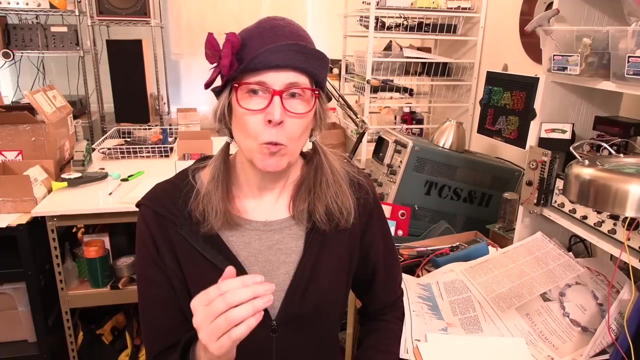 I hope I don't have to turn off comments for this video, but, in a nutshell, the beautiful thing about climate change is that it doesn't care if you believe in it or not, And so if you don't believe in climate change, watch something else. But for those of you who care about this, let's really examine, first of all, why there is even a controversy about 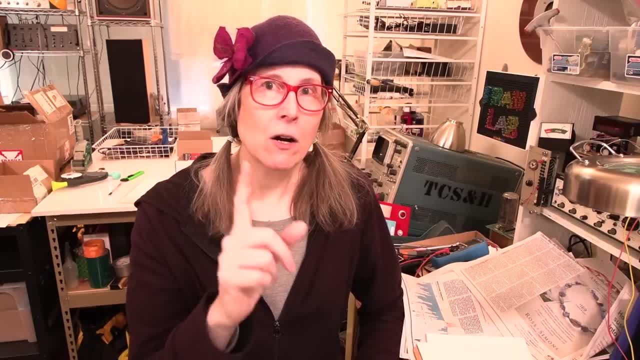 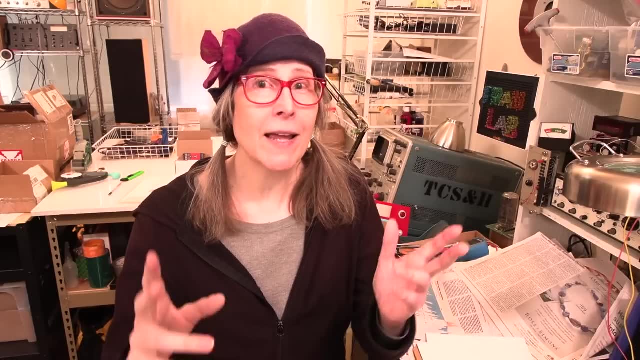 CO2.. And in a larger sense I'm going to say carbon in the atmosphere. I've done videos before where I talk about carbon in the atmosphere and there's a you know a- flood of comments. Fran, you're not being scientifically correct. You're not following the science. It's not carbon. people saying carbon It's not carbon, It's carbon dioxide. 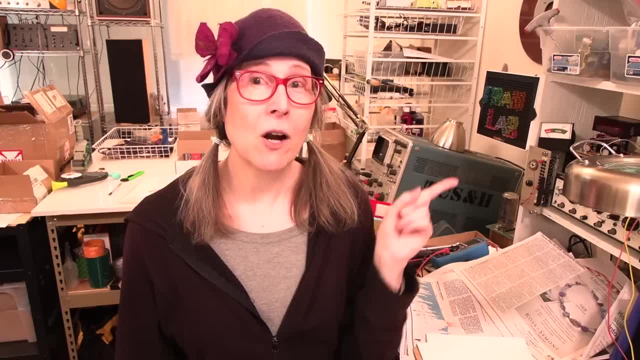 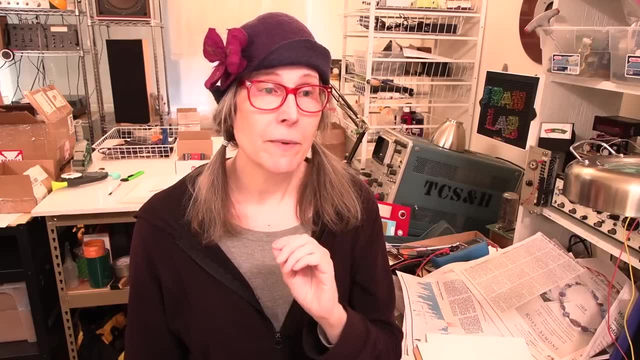 CO2, Fran It's called CO2, carbon dioxide, not carbon. That's not true. It's carbon in the atmosphere. Any gaseous molecule that is based on carbon, That's carbon dioxide. carbon monoxide, methane. 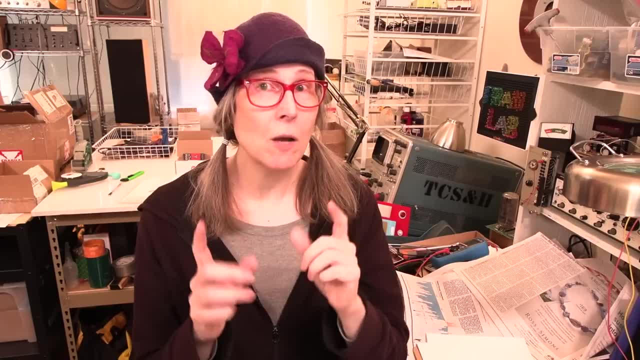 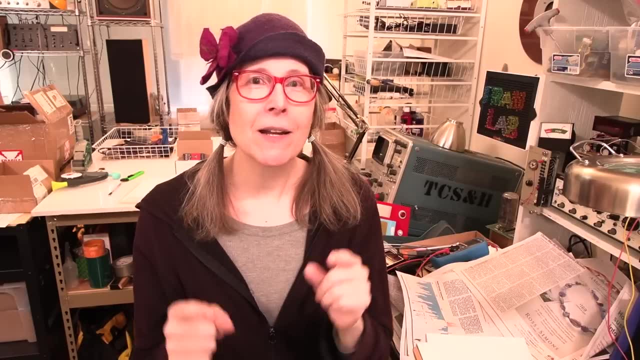 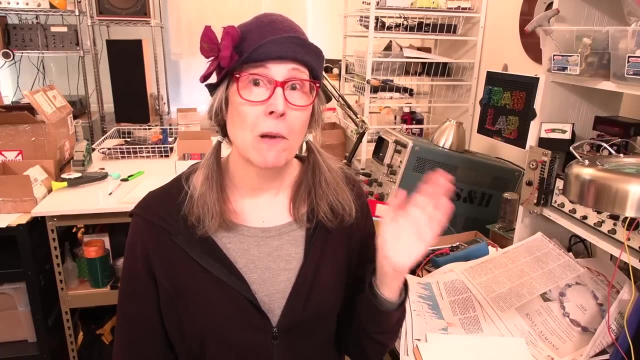 There are lots of these greenhouse gases. They're all based on carbon. Any molecule that is in the atmosphere that is based on a carbon atom is part of the problem, CO2 being by far the largest of those. but all those carbon-based molecules, they all have some effect on the greenhouse effect. 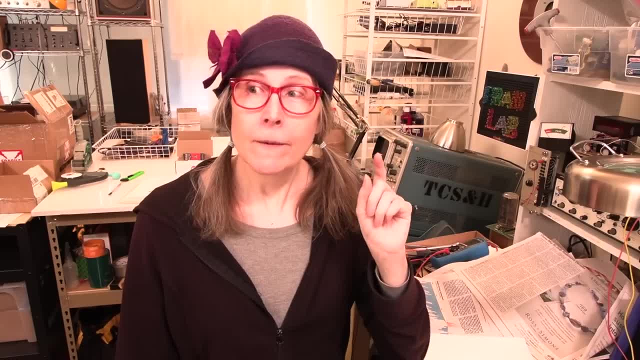 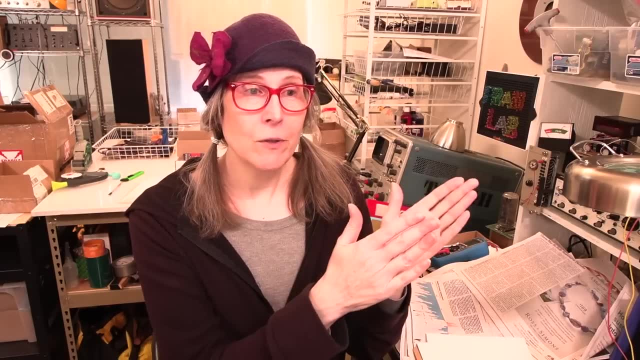 in dealing with climate change. So the number one obstacle in whether or not people even accept the argument about climate science: it comes down to those who have some understanding of how much carbon dioxide is actually in the breathable atmosphere and those that don't, and don't really care. 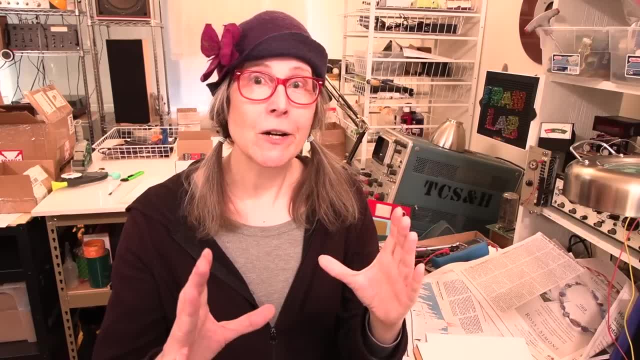 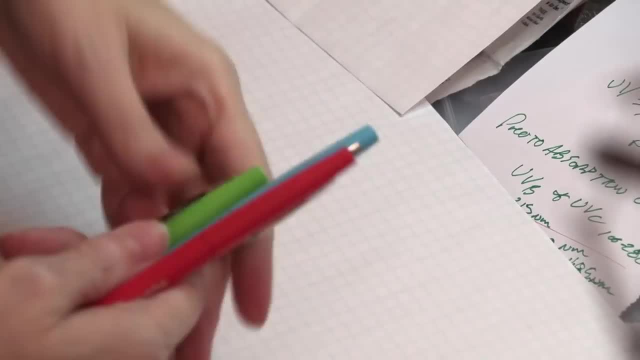 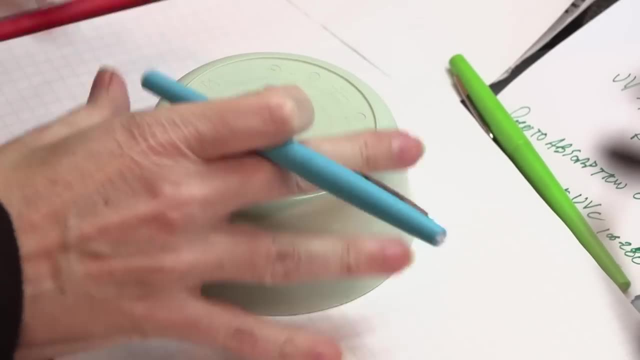 Let's look at our atmosphere in a pie chart and see really what we're breathing in. anyway, All right, so let's get my handy pie chart maker and yeah, so let's say: let's see what we've got here. 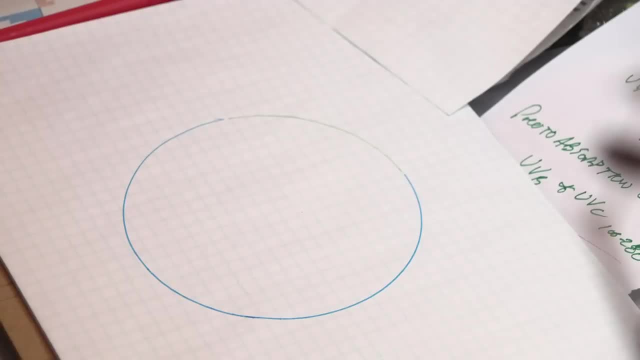 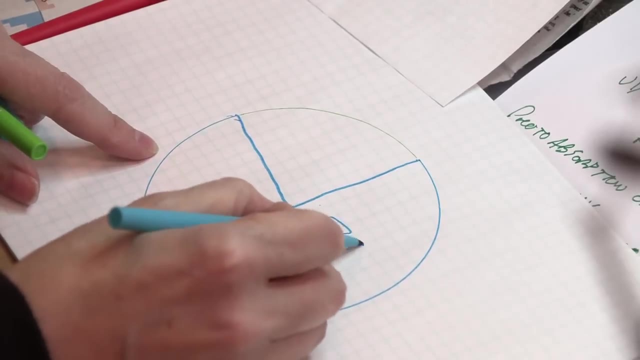 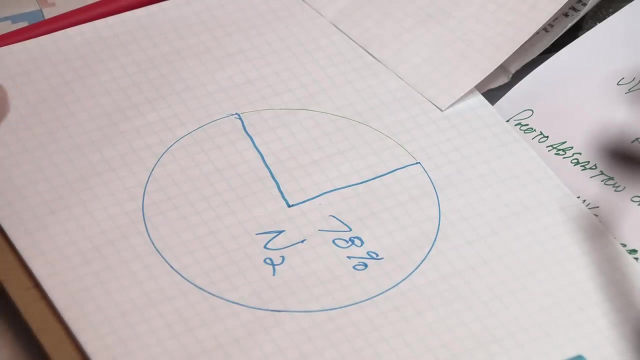 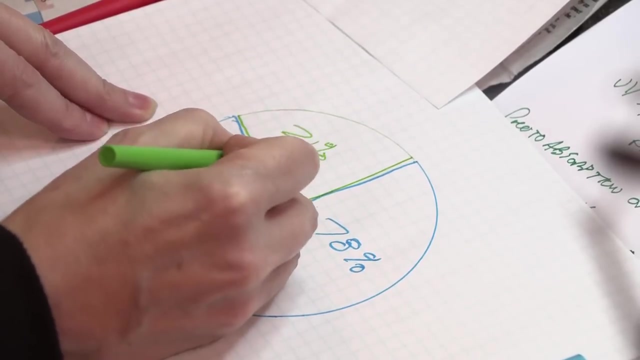 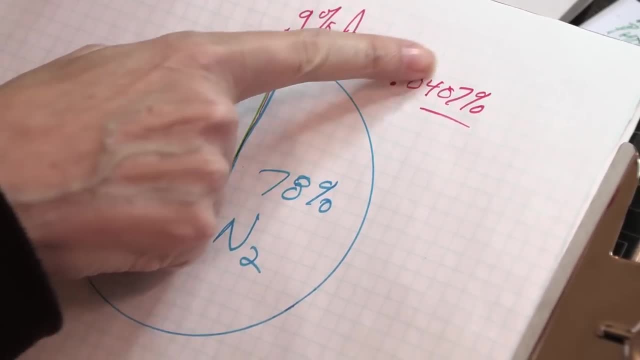 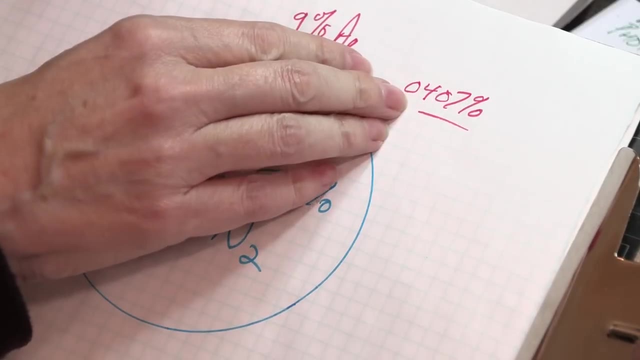 That's four one-hundredths of a percent. and change of the atmosphere: Four one-hundredths of a percent. carbon dioxide- A minuscule concentration When you look at this number, if you're thinking of the pie chart of the atmosphere. 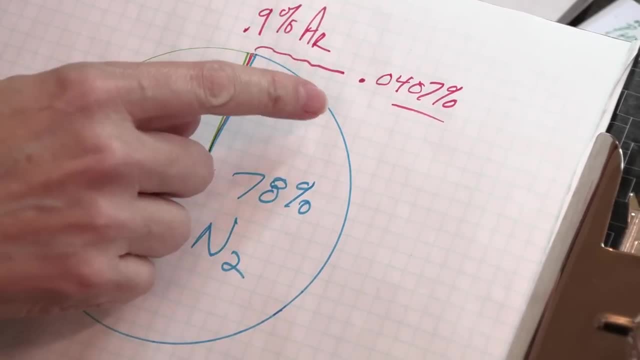 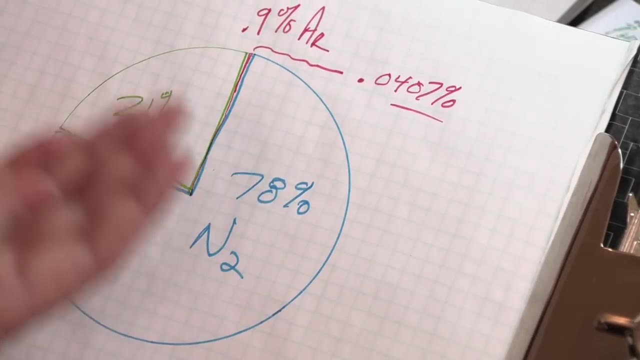 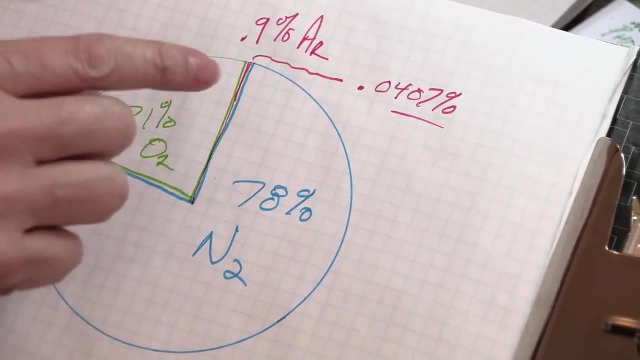 why is it hard to think that 200 years of industrialization, burning coal, burning gas, automobiles, jet planes, all of the carbon that we churn into the atmosphere, all of the carbon that we churn into the atmosphere every year, and orders of magnitude more and more every decade, 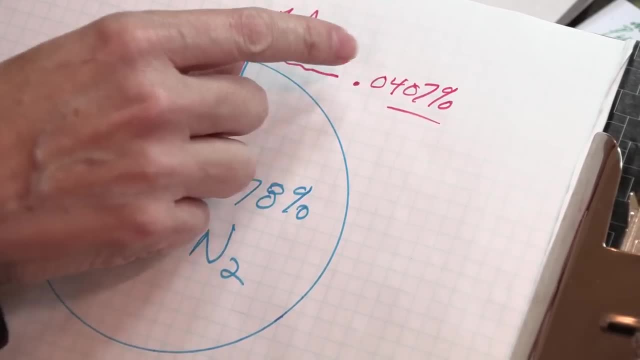 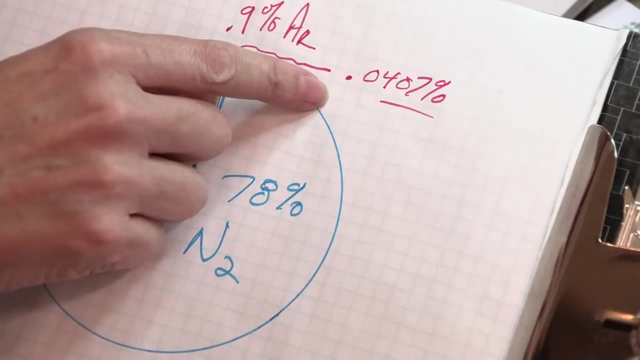 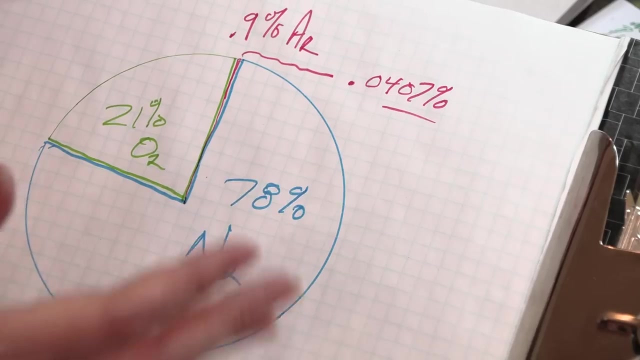 why would we think that changing that number is impossible And why would we think that, with a greenhouse gas, that minuscule changes, the concentration of which will have changes in the global temperature in the degrees, would make a difference? Well, that's really the basis of client science. 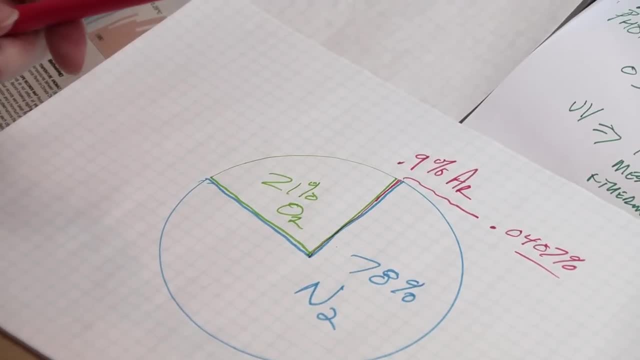 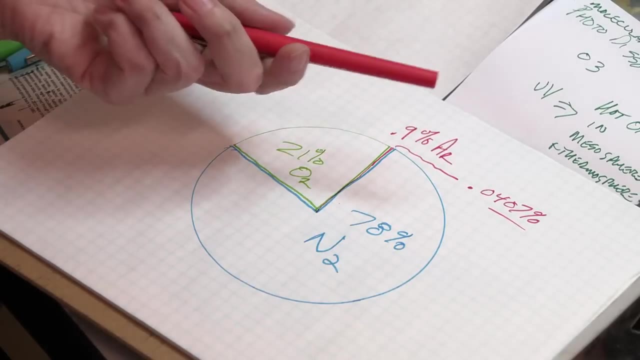 It doesn't really matter for the planet what the concentration of CO2 is. Earth doesn't care what the concentration of CO2 is. In fact, it talks with its sister planet, Venus, all the time, and Venus doesn't complain about CO2.. 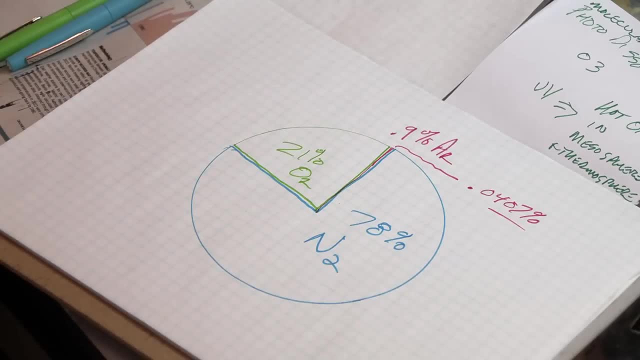 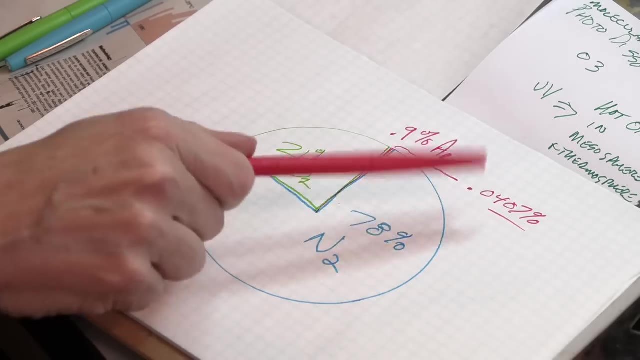 Venus says: hey, you know I love CO2.. If it weren't for CO2, I wouldn't have like a thousand degree temperatures on my surface. So yeah, the greenhouse gases, CO2, methane, carbon monoxide. 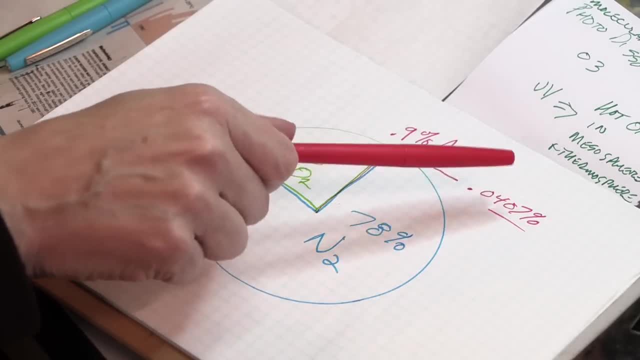 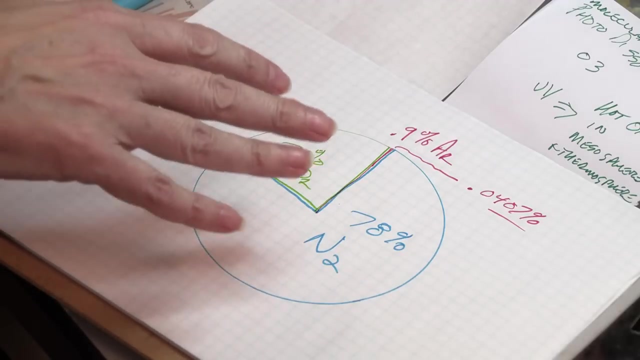 all the carbon compounds that we end up putting into the atmosphere artificially. it has huge ramifications for our species because we like the planet the way that it is. We don't want it to be two, three, four degrees hotter. We like the sea levels where they are because we build our cities and our towns right up to them. 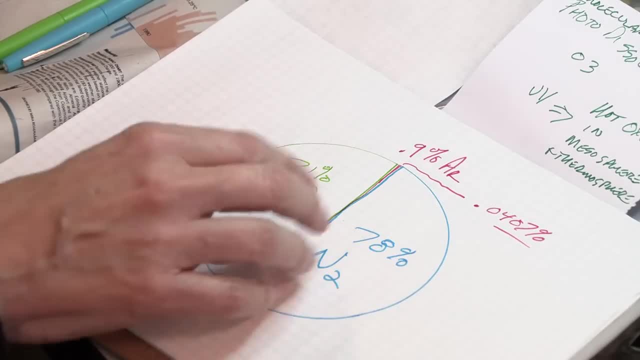 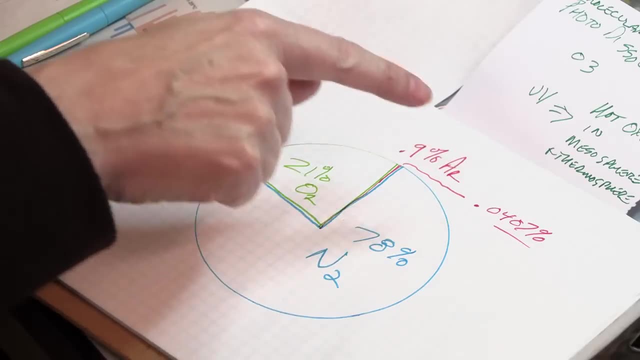 so we don't want them to be higher. Yeah, so it's in our best interest to lower that number a little bit, to get it down to pre-industrial levels and pre-industrial concentrations of CO2.. We have other hard choices to make. 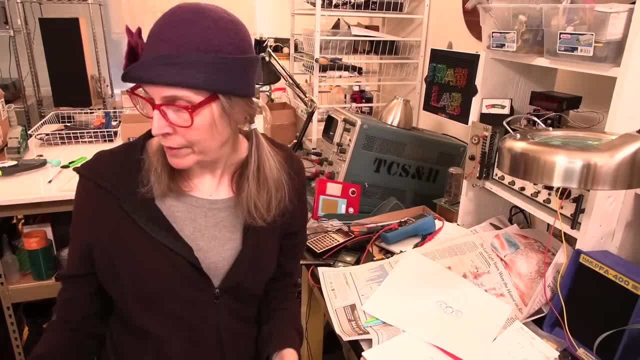 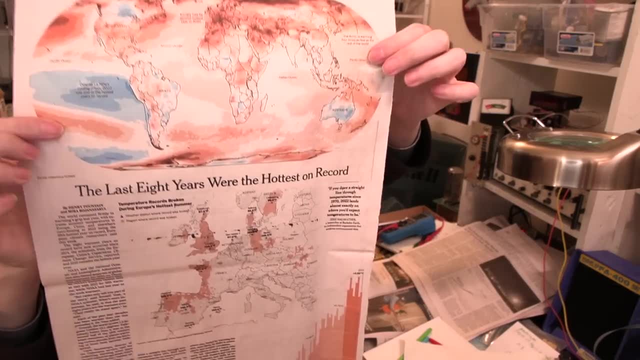 Because as great as the headlines are for the ozone layer coming back, the headlines for CO2 are not so great. you know, The last eight years were the hottest on record. You know, if you want data, you can get it. if you really want data, 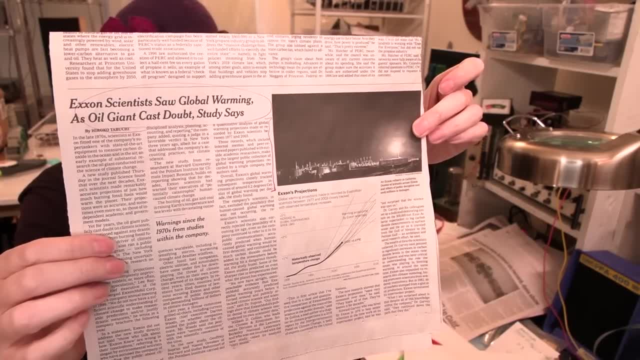 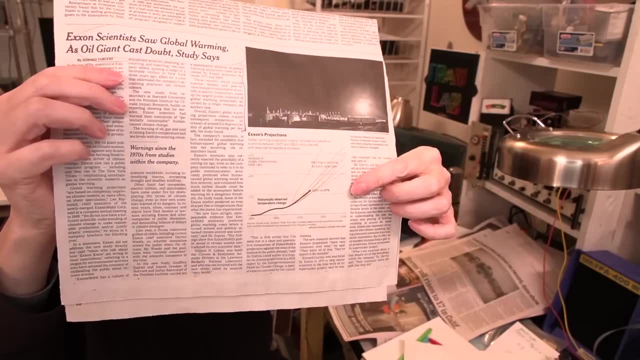 Exxon scientists saw the global warming coming as oil giant cast doubts. A study shows about how Exxon had their own scientists revealing that they knew that the increase in CO2 was going to be higher. They said: you know carbon dioxide and other carbon compounds were going to change the atmosphere. 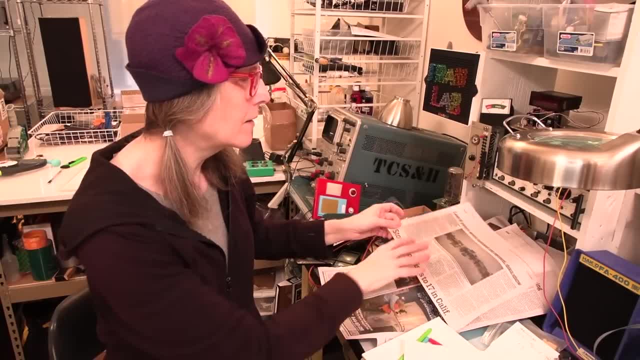 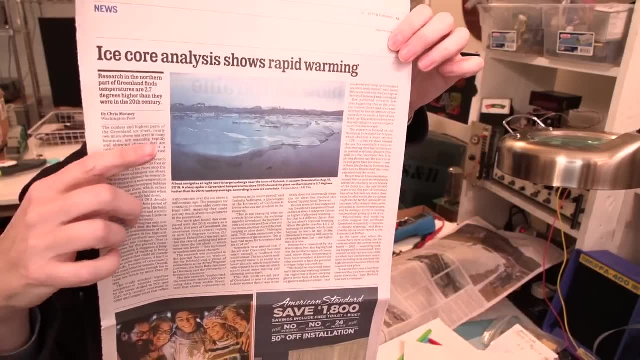 and their predictions pretty much landed on exactly what happened. but they didn't care. The last eight years were the hottest on record Data show another one: Ice core analysis in Greenland shows rapid warming. In fact, Greenland is one of the fastest warming places on the planet. 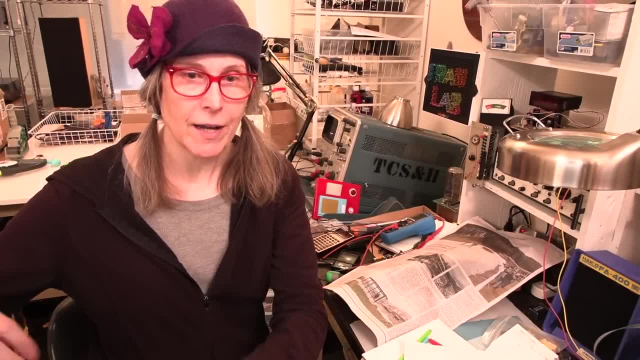 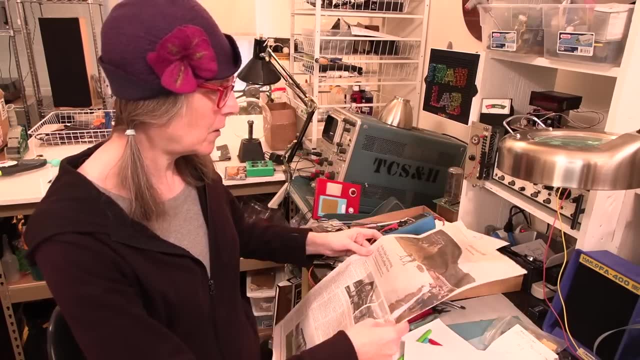 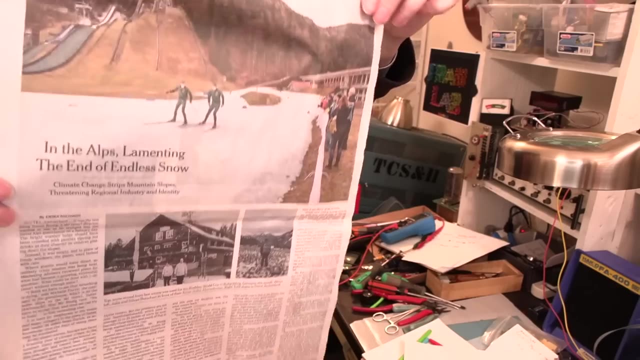 and contains, like most of the freshwater, ice. Why should we care if Greenland melts? Well, you know, if you like your cities where they are, you ought to care And even like impact on commerce. The Alps lamenting the end of endless snow. because even in the Alps, no snow. 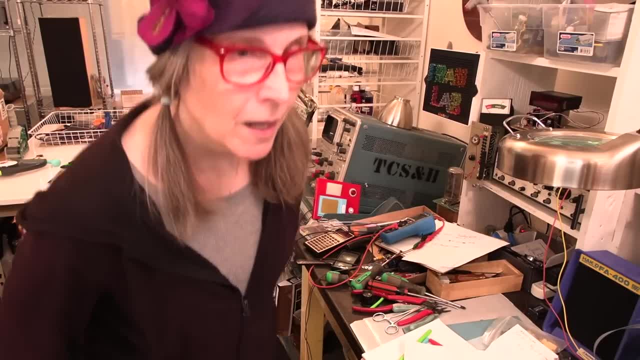 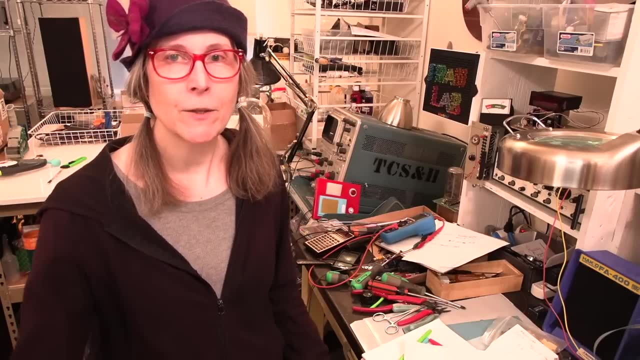 So it goes on and on and on, of course. But you know, when you talk about climate, you're either preaching to the converted or you're, you know, screaming into the vacuum. But you know, I think that the ozone data is a good sign. 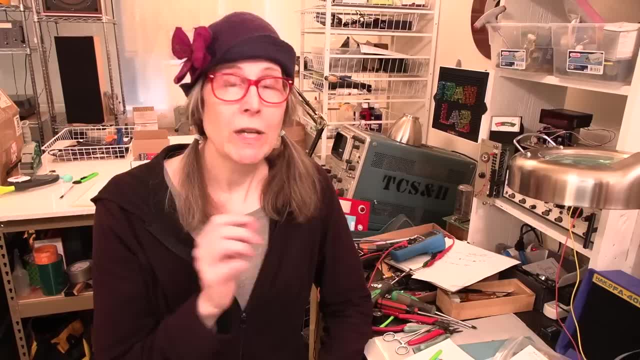 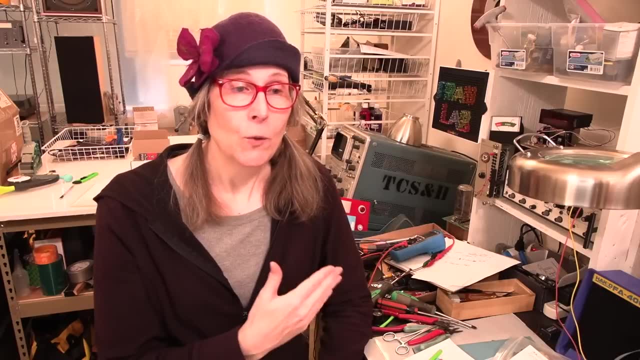 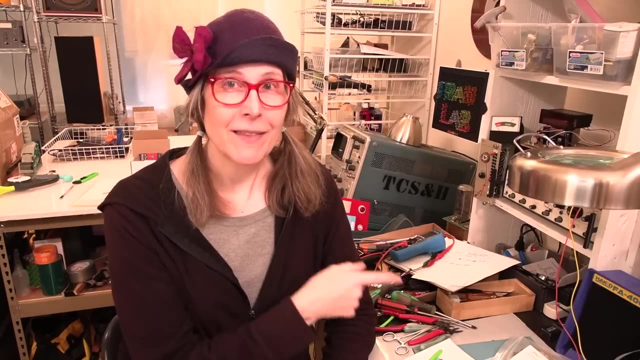 It shows that we can make decisions as a species to change the way that we do things in a way which, at the front, makes a lot more work and a lot more cost because replacing CFCs. there were a lot of people that protested that. because CFCs were cheap, easy, readily available and nonreactive, And so finding chemicals to replace refrigerants that we had used for decades and pressurants that we used for decades, that was costly. The new stuff cost more and it wasn't as effective. 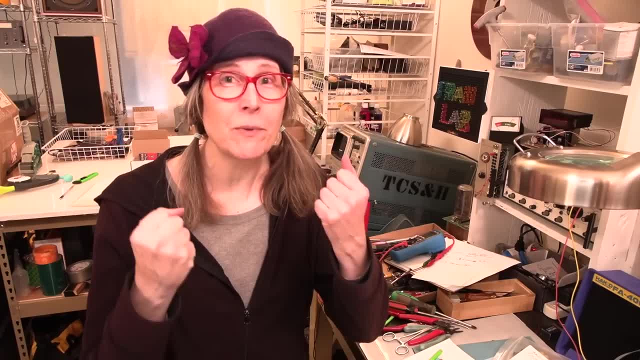 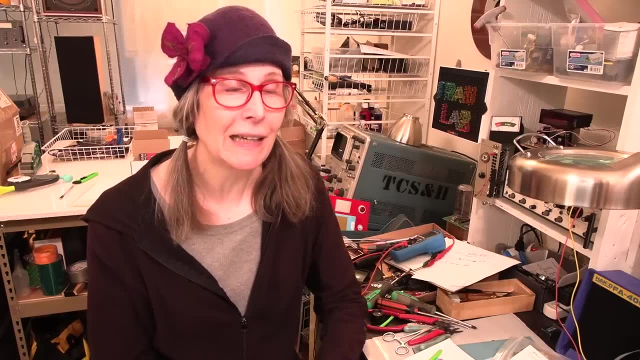 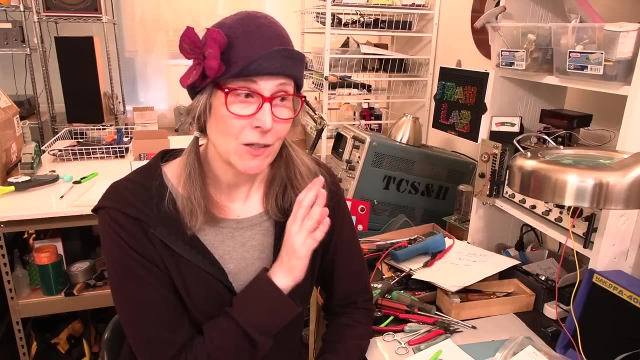 It couldn't be compressed as much, It couldn't store as much energy in it. People still complain about it, But we made those tough choices because we realized that we didn't want to be cooking under UVB. Yeah, so climate change is just another thing where, with CO2 and carbon compounds, we've been messing up for a lot, lot longer than CFCs. So many orders of magnitude more CO2 and methane and other compounds than CFCs. Yeah, we've been messing up for a lot longer than CO2 and methane and other compounds. 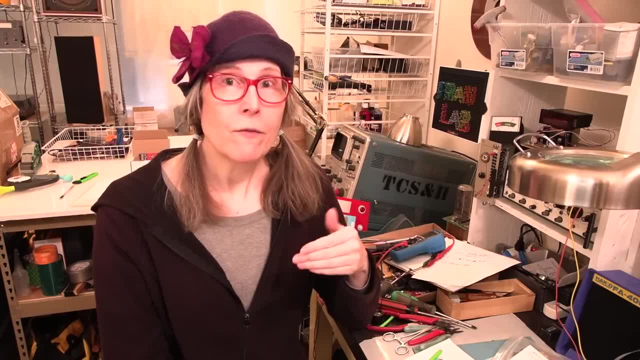 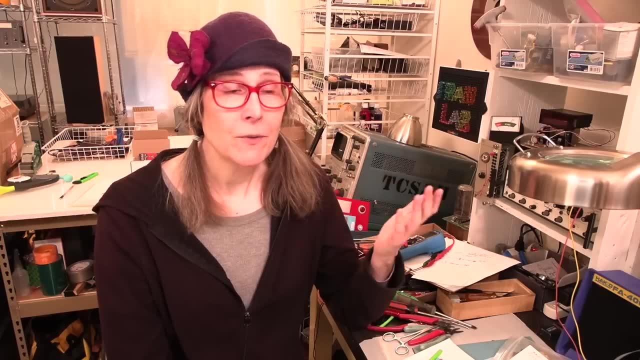 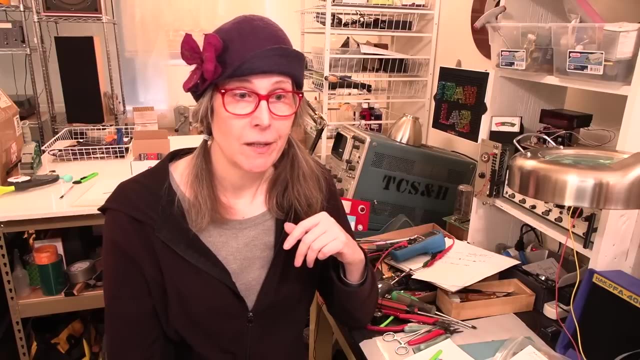 than we ever did chlorofluorocarbons. But even with going off fossil fuels, it is possible for us to do that. We can do that, We can make those decisions And although the difference between the ozone layer, where we could possibly have it repaired to pre-industrial levels before the century, is out, 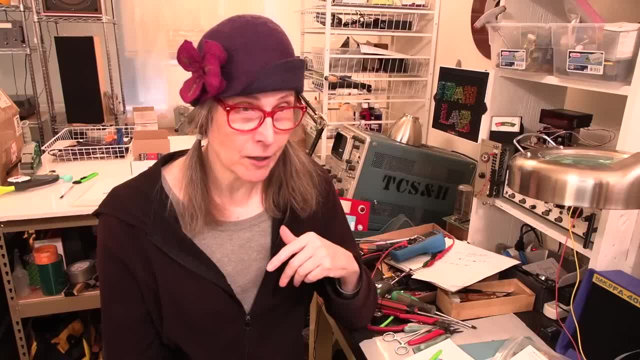 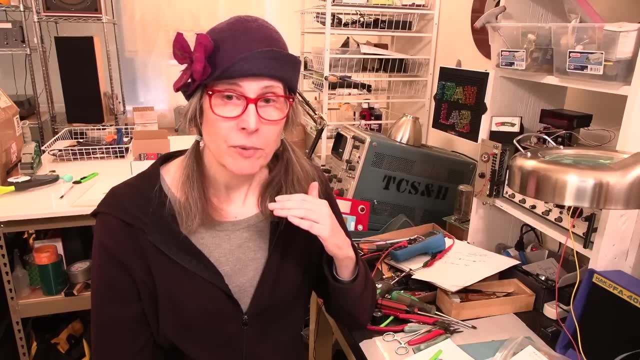 with climate change, we've set in motion something that's going to take a lot longer for natural processes to reverse. The best we can hope for with climate change is to arrest our production of carbon dioxide and other greenhouse gases to basically level it off. 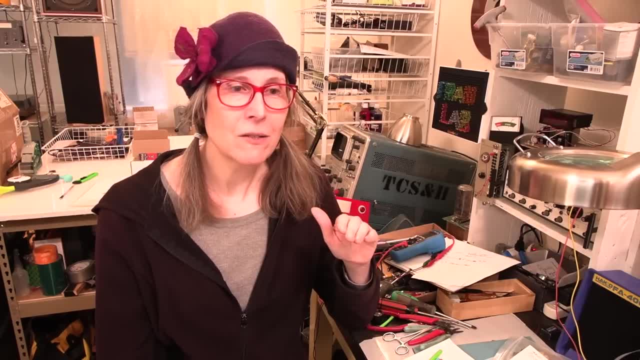 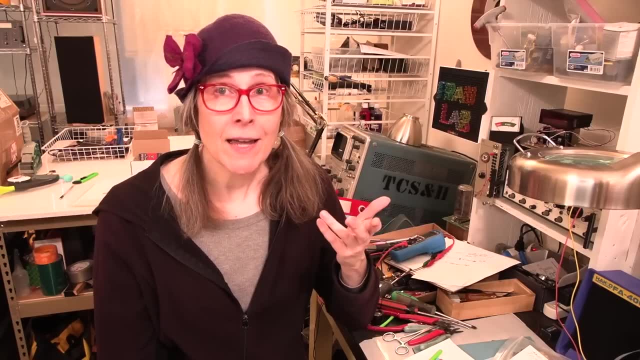 That's one hurdle. The next is to stop producing so much greenhouse gas so that we can allow the natural processes to slowly reverse it. And then even then, at this point, we're still going to have to make hard choices to change the way that we live. 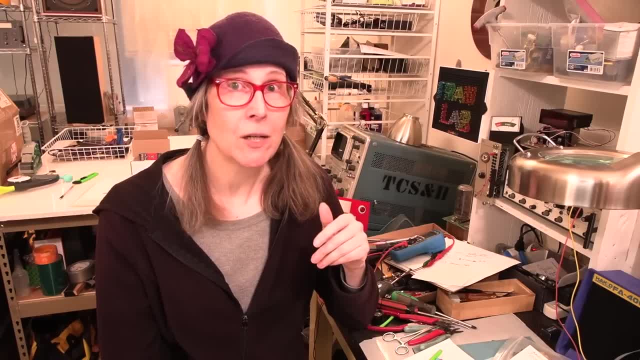 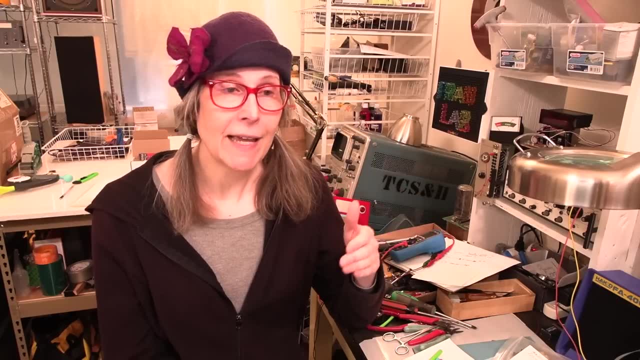 so that we can endure a much hotter planet for, you know, possibly centuries- As we figure out how to change the ways that we grow plants and use land and produce energy and other resources. we're going to have to make lots of hard decisions. 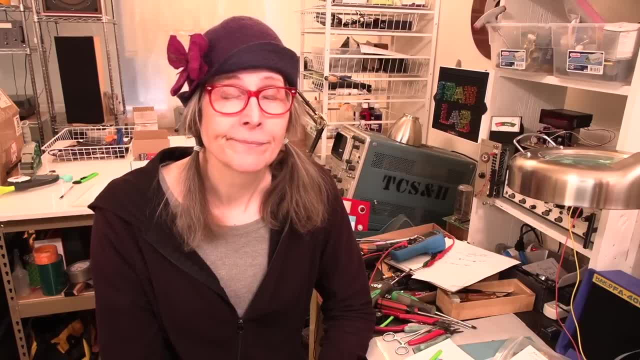 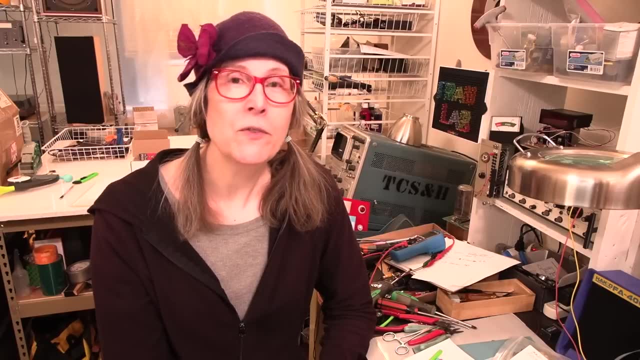 and make lots of changes, And people hate change. It's the number one thing that makes people lose their minds is the idea of change, And we are in a time of change, so people are losing their ever-loving mind. The people screaming the loudest. 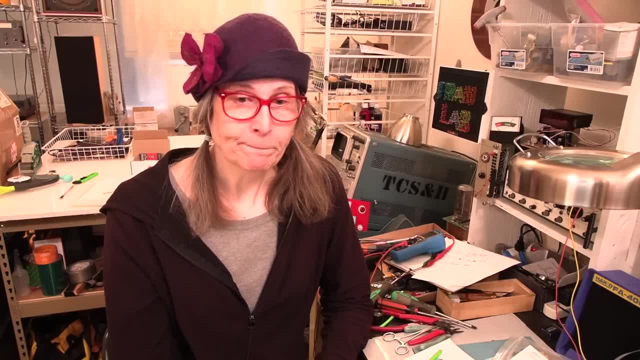 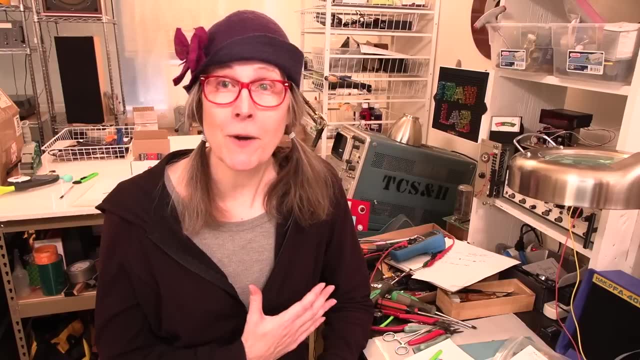 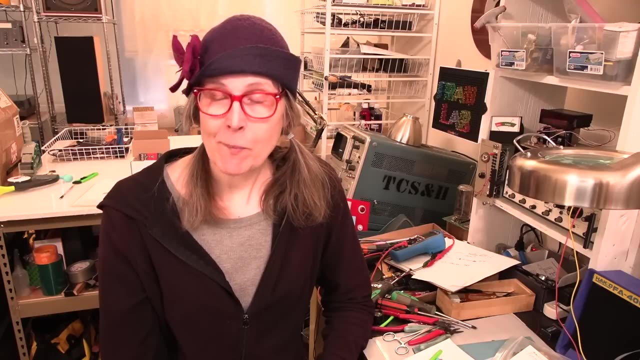 are always the people who fear change the most, But these decisions, like all decisions that we make, are completely up to us. The ozone layer: good news. It would be interesting that perhaps in my lifetime that we could even get better news on the ozone layer. 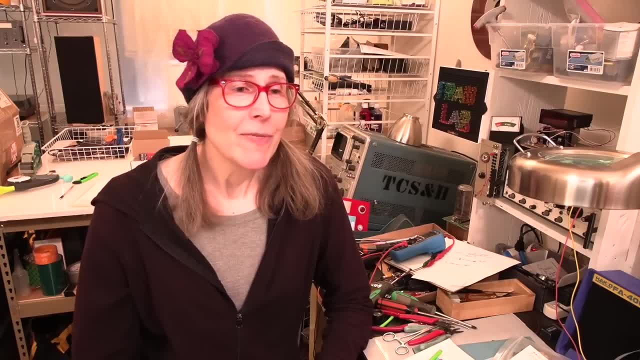 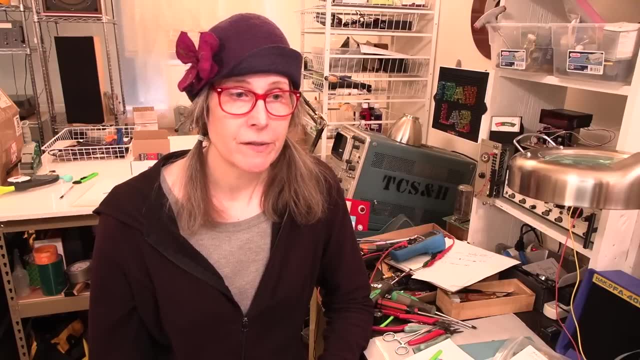 But as far as the global warming is concerned, that is an arc that's going to take a long, long time, even with our best efforts, centuries, to have a change for the better. That's it for this one, a long one. 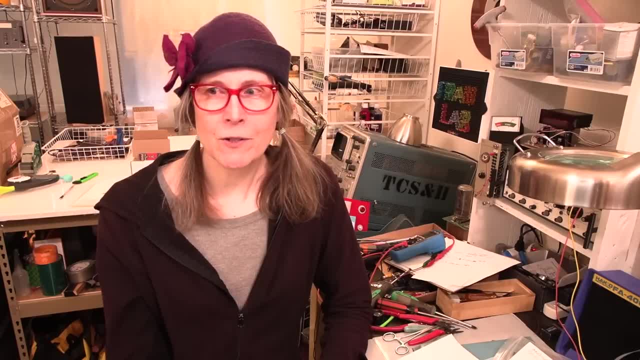 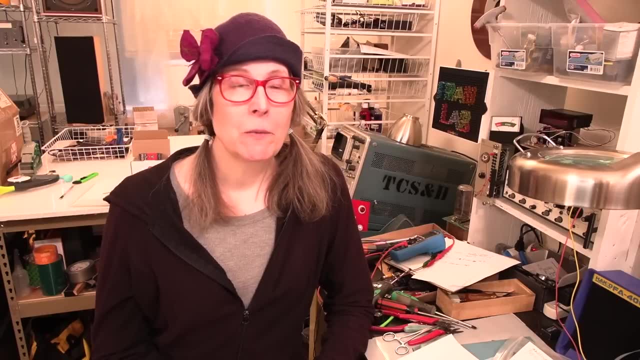 and I talked a lot. I hope I don't have to turn off comments because people just go nuts. It's just the crazies, But that's what happens. You know, we don't teach chemistry anymore. How many people really have a functioning knowledge? 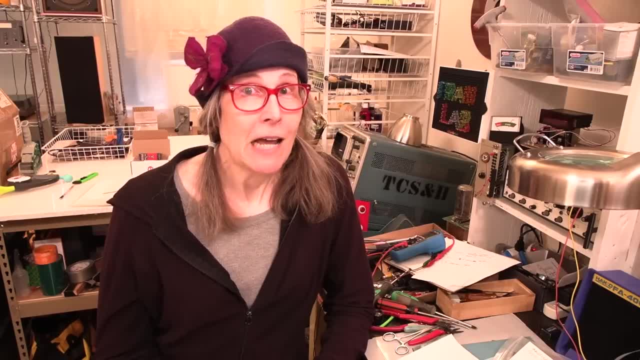 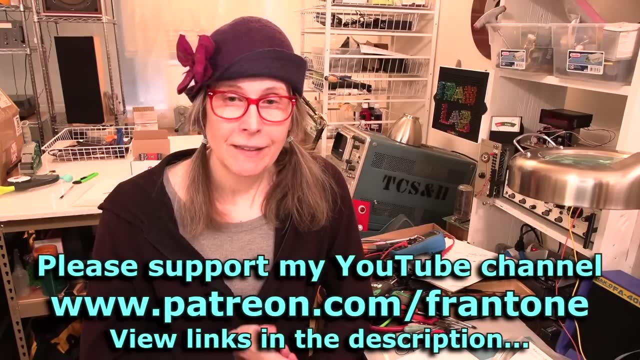 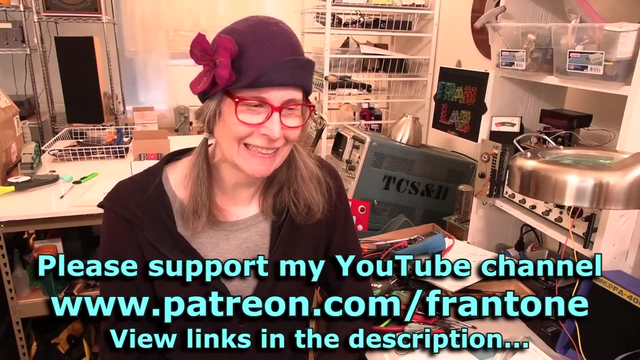 of real chemistry these days: Not many, Not many. But yeah, chlorine, our favorite halogen, is on the decline in the stratosphere and we're very grateful for that. But it wasn't for a lack of trying. All right, I'm Fran. 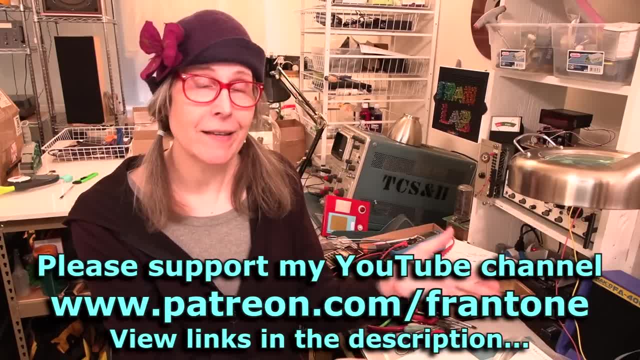 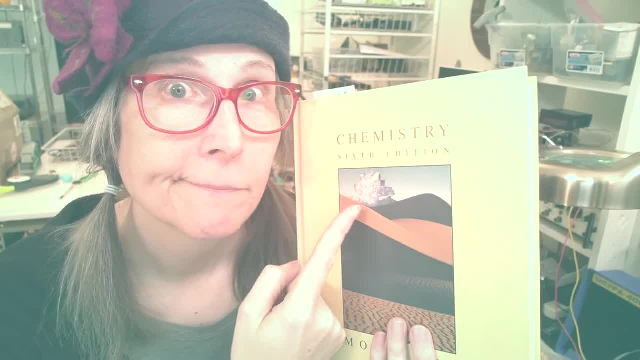 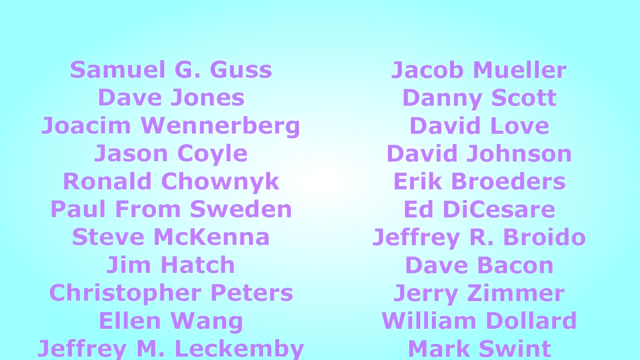 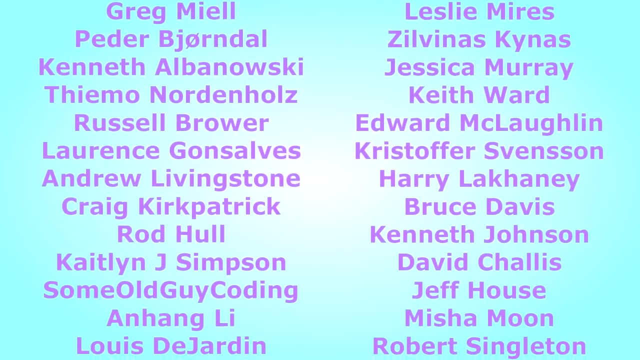 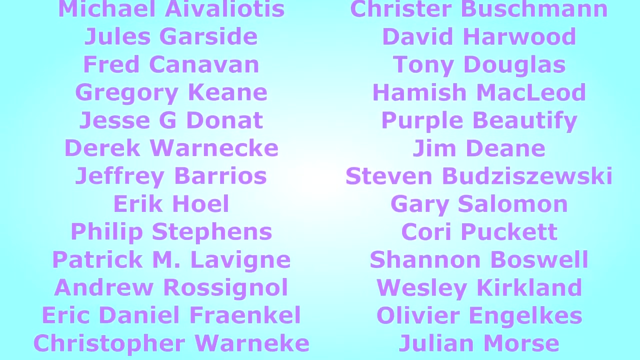 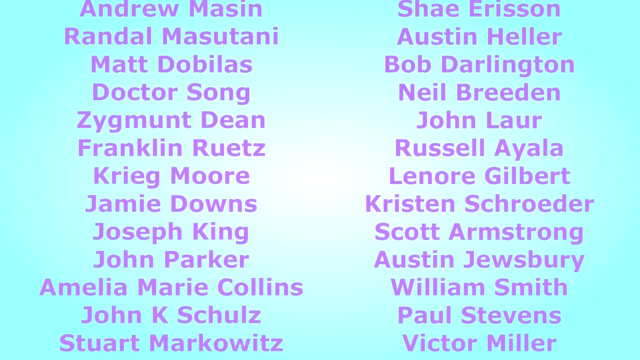 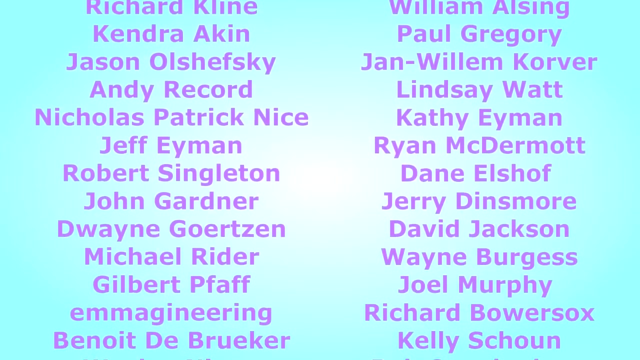 I'll be back here at the bench doing something else, science-y, real soon. Bye, I'm gonna laugh. That's where I work In the lab. Go berserk In my lab. That's where I work For you and me. 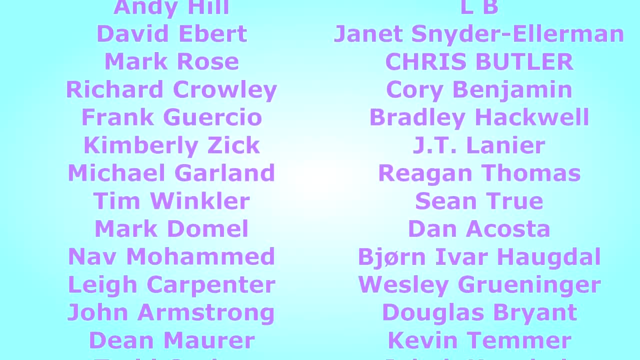 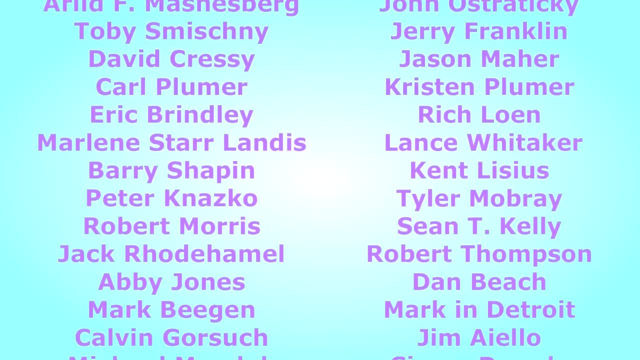 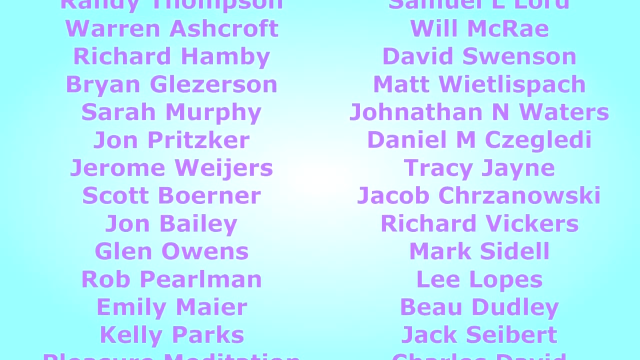 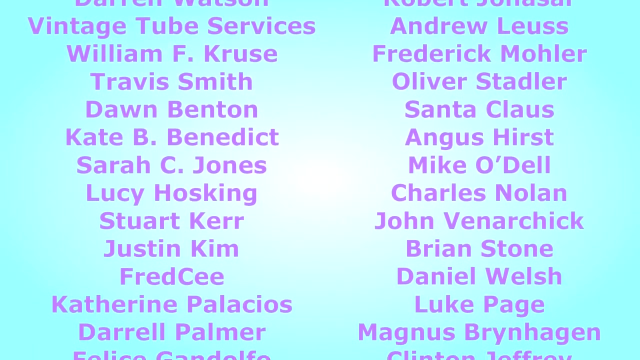 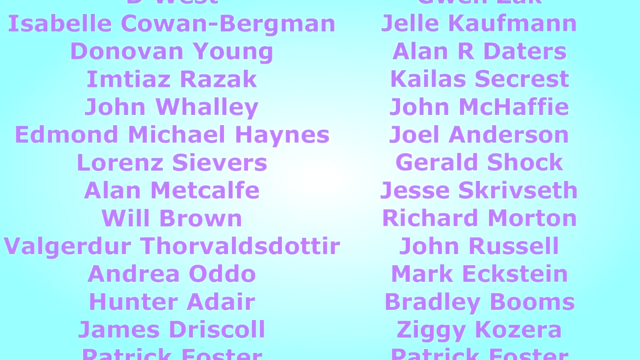 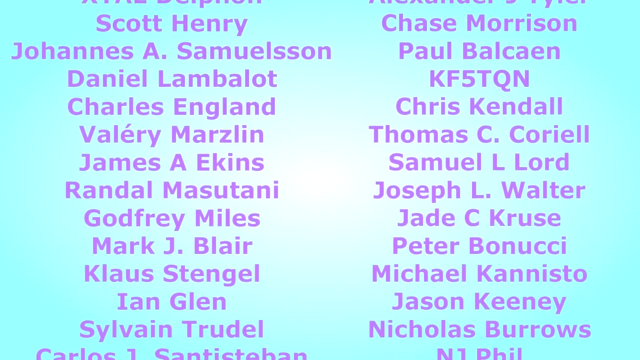 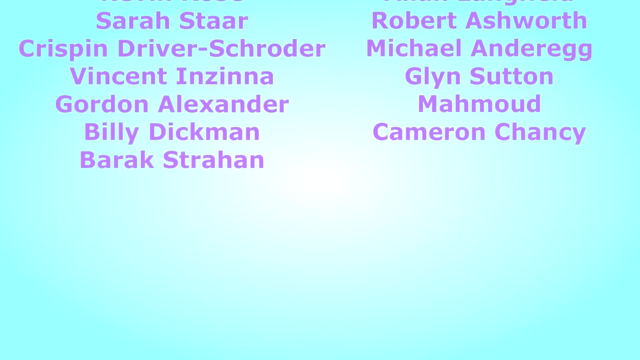 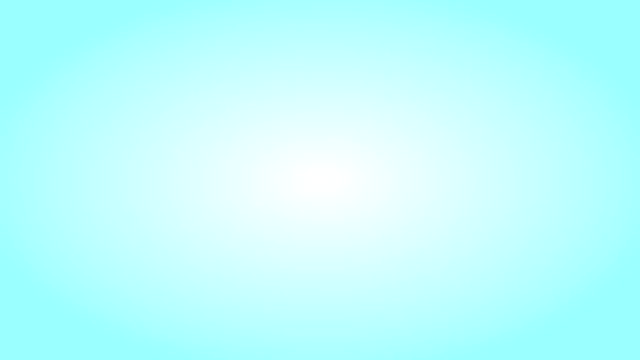 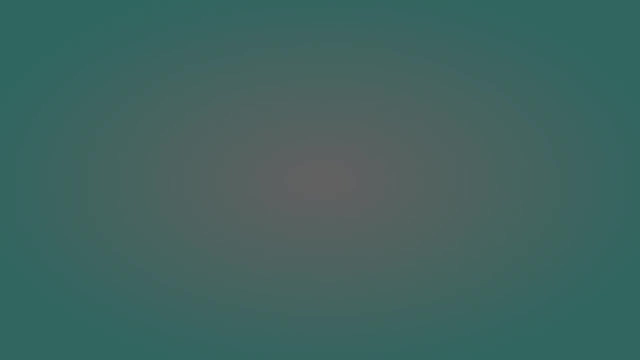 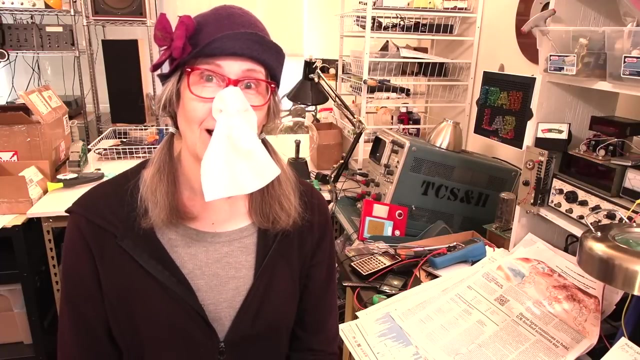 bones and hearts. music, ukulele, music, music, music, music. It's what you're watchin', Friend, love, It's what I'm doin' Workin' at the bench. Again, I'm Fran. I'm Fran, Never gets old.